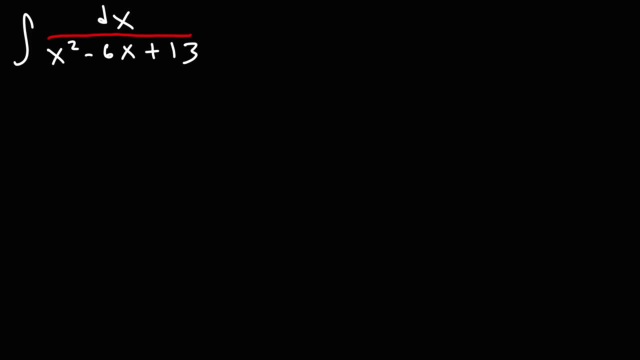 Consider the problem on the screen. What is the antiderivative or the indefinite integral of dx over x, squared minus 6x plus 13?? How can we find this answer? Well, we need to integrate it by completing the square. But before we do that, there are some. 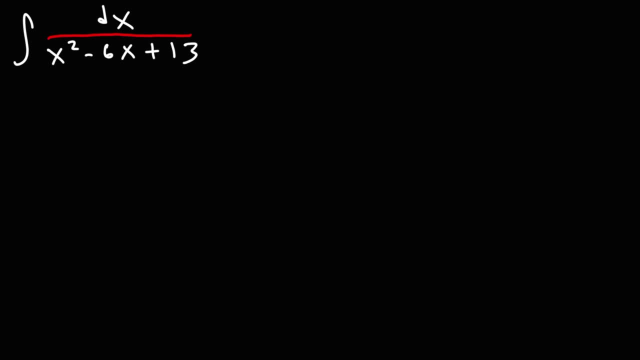 formulas that you need to know for problems like this, So you may want to write this down. The first one is this one: The integral of du over a squared plus u squared, That's 1 over a. r tangent u over a plus c. a is a constant, u is a variable, u is basically a function of x. 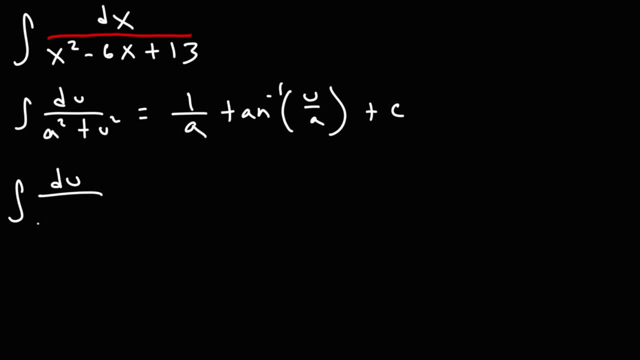 The second one is this one, The integral of du, over the square root of a squared minus u squared, And this is equal to arc sine u over a plus c. Now, the next one you want to be familiar with is this one: The integral of du. 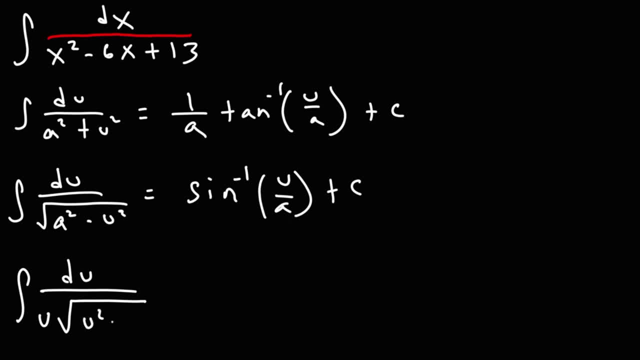 divided by u square root, u squared minus a squared, And this is equal to 1 over a arc, secant absolute value of u over a plus c. Now looking at our problem: which of these three formulas should we use for this problem? 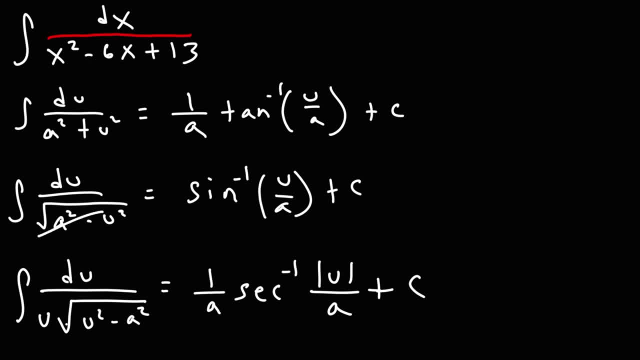 Well, it's not going to be arc sine or arc secant, because we don't have a square root, So likely it's going to be arc tangent. Therefore, we need to complete the square in order to put it in this form. 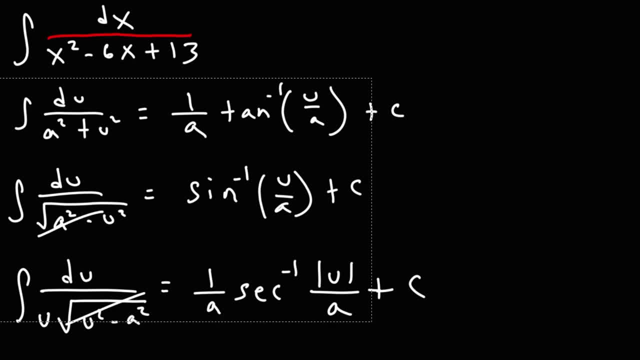 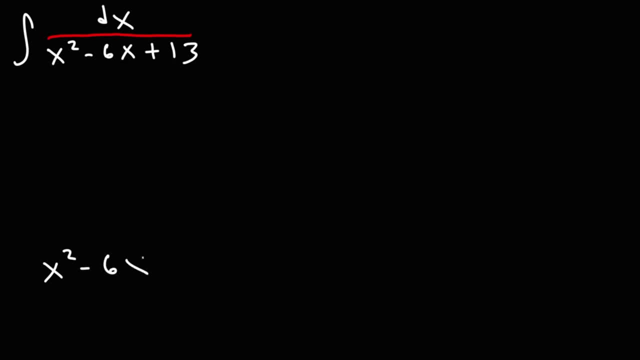 So let's go ahead and do that. We have x squared minus 6x, plus 13,, which I'm going to rewrite it as x squared minus 6x, And then I'm going to leave a space plus 13.. In order to complete the 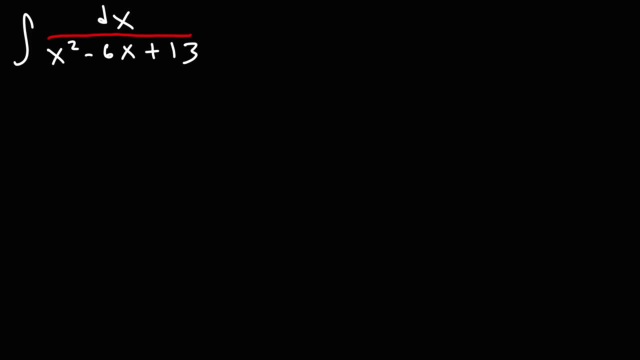 Consider the problem on the screen. What is the antiderivative or the indefinite integral of dx over x, squared minus 6x plus 13?? How can we find this answer? Well, we need to integrate it by completing the square. But before we do that, there are some. 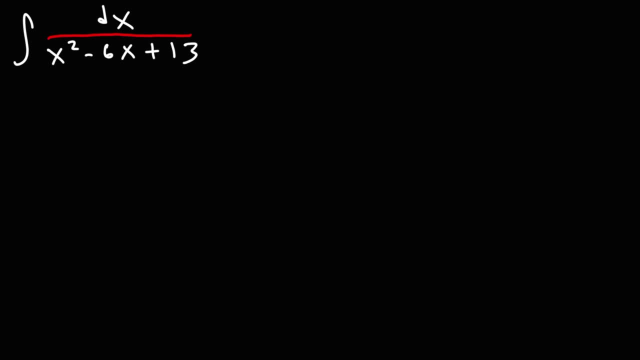 formulas that you need to know for problems like this, So you may want to write this down. The first one is this one: The integral of du over a squared plus u squared, That's 1 over a. r tangent u over a plus c. a is a constant, u is a variable, u is basically a function of x. 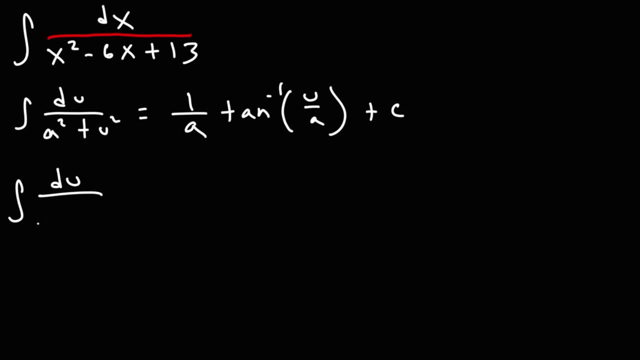 The second one is this one, The integral of du, over the square root of a squared minus u squared, And this is equal to arc sine u over a plus c. Now, the next one you want to be familiar with is this one: The integral of du. 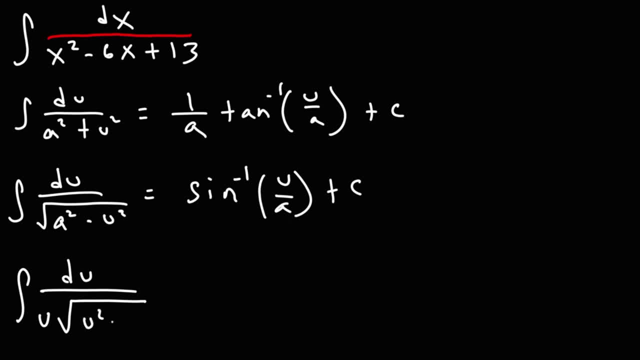 divided by u square root, u squared minus a squared, And this is equal to 1 over a arc, secant absolute value of u over a plus c. Now looking at our problem: which of these three formulas should we use for this problem? 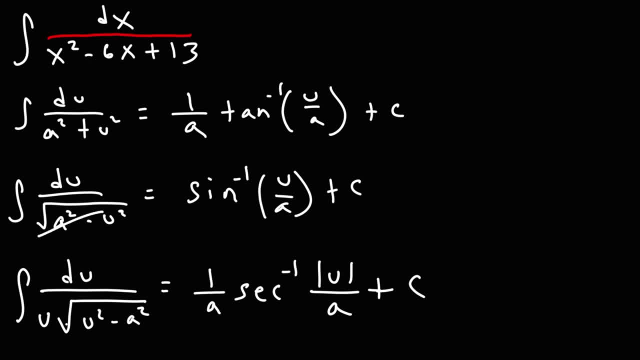 Well, it's not going to be arc sine or arc secant, because we don't have a square root, So likely it's going to be arc tangent. Therefore, we need to complete the square in order to put it in this form. 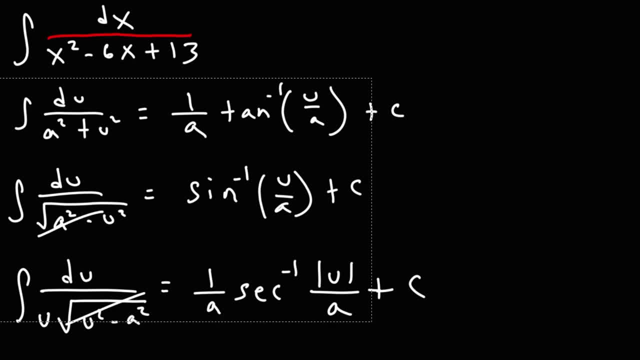 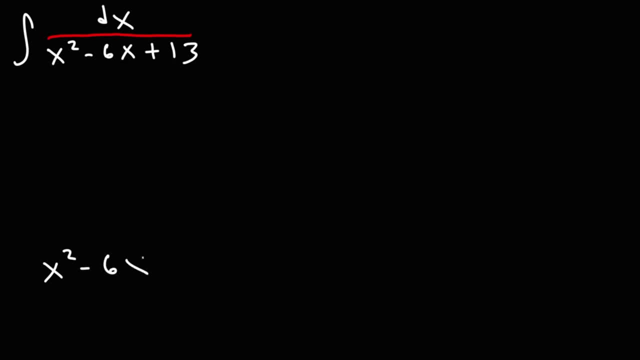 So let's go ahead and do that. We have x squared minus 6x, plus 13,, which I'm going to rewrite it as x squared minus 6x, And then I'm going to leave a space plus 13.. In order to complete the 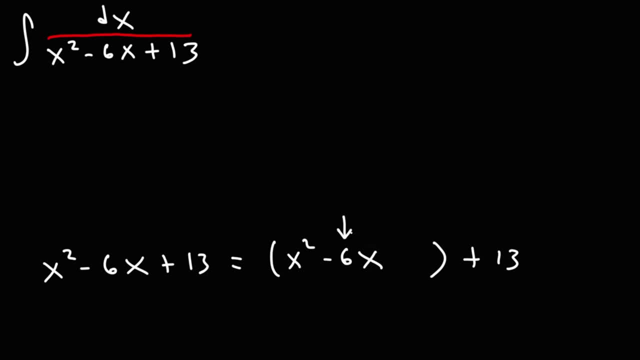 square. focus on this coefficient, the number in front of x. Don't worry about the negative sign for now. So take half of that number- half of 6 is 3, and then square it. So we're going to add 3 squared. 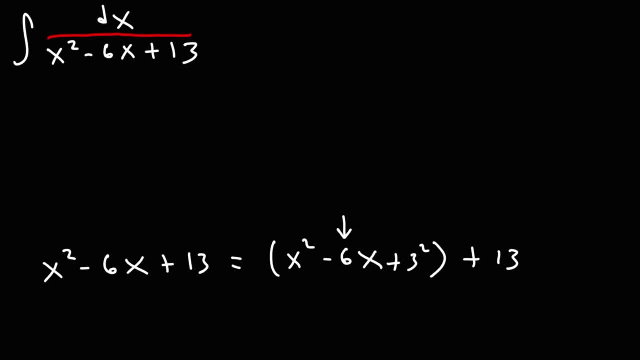 which is equivalent to 9.. Now, because we've added 9 to this expression, we've changed the value of that expression. In order to maintain the value of that expression, we need to undo this over here. So, because we added 9, we need to subtract 9.. By doing that, we maintain the value. 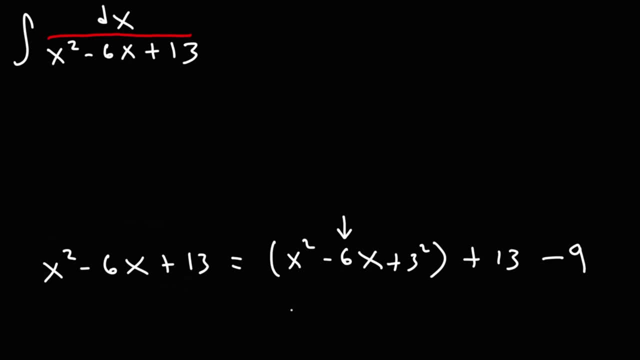 of this expression. So now what we have here is a perfect square trinomial, And we could factor it like this: So it's going to be x, whatever this sign is minus, and then what we see here: 3 squared. 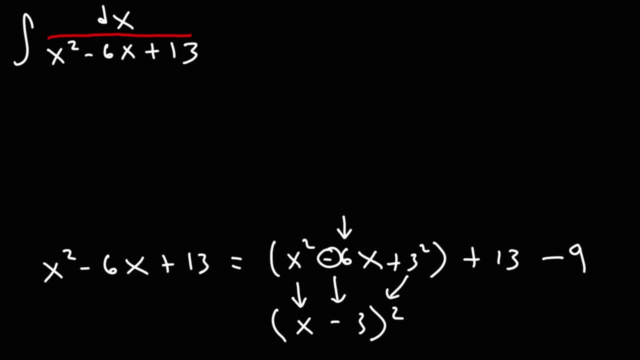 That's a quick and simple way to factor a perfect square trinomial. Here we have 13 minus 9, which is 4.. So this is going to be dx, Or the integral of dx, over x minus 3, squared plus 4.. 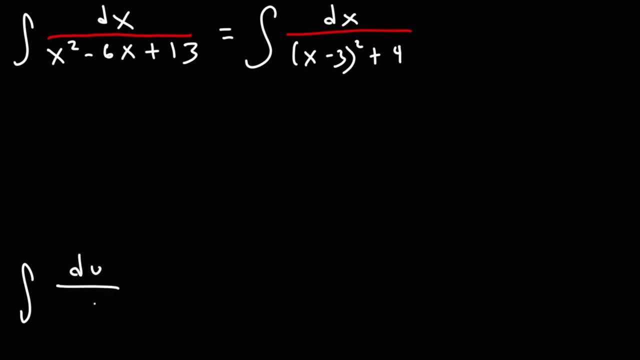 So notice the form that we have it in. We almost have it in this form, But we're not quite there yet. What we're going to do is we're going to make u equal to x minus 3.. By doing that, du is going to be the derivative of x minus 3, which is 1.. 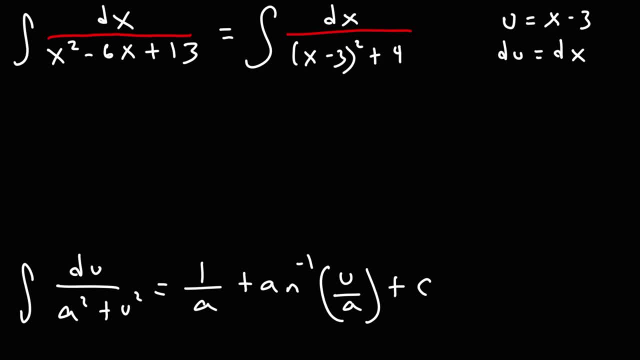 The derivative of x is 1, but 1dx. So du is equal to dx. So we can replace x minus 3 with u And we're going to have plus 4.. So u squared over 4.. Therefore we could see that a squared is equal to 4.. 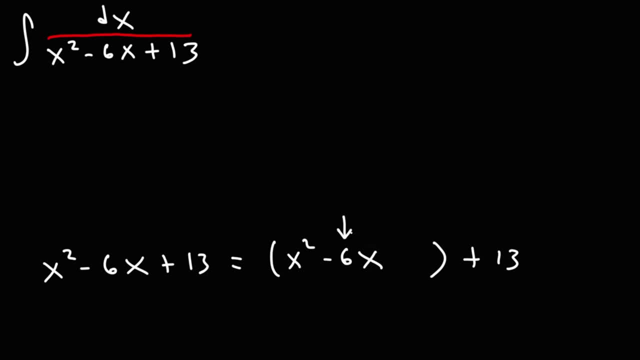 square. focus on this coefficient, the number in front of x. Don't worry about the negative sign for now. So take half of that number- half of 6 is 3, and then square it. So we're going to add 3 squared. 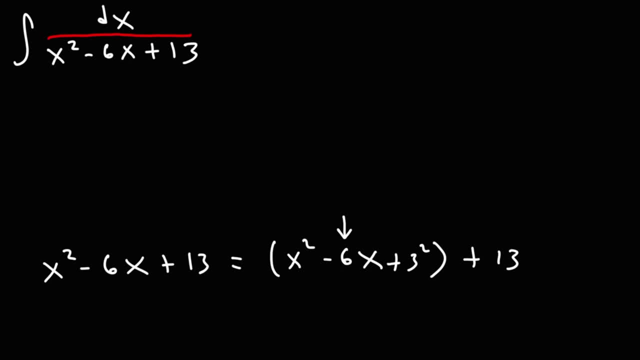 which is equivalent to 9.. Now, because we've added 9 to this expression, we've changed the value of that expression. In order to maintain the value of that expression, we need to undo this over here. So, because we added 9, we need to subtract 9.. By doing that, we maintain the value. 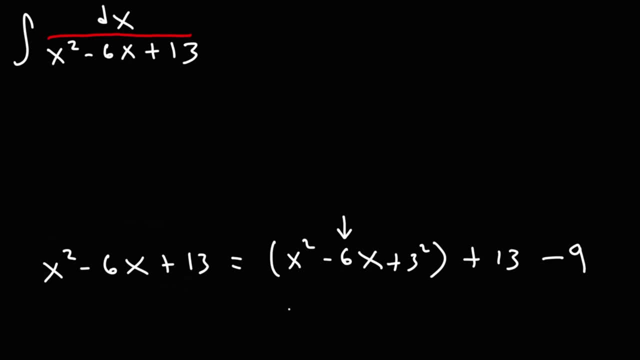 of this expression. So we're going to add 3 squared, which is equivalent to 9.. And then we're going to: So now what we have here is a perfect square trinomial, And we can factor it like this: So it's: 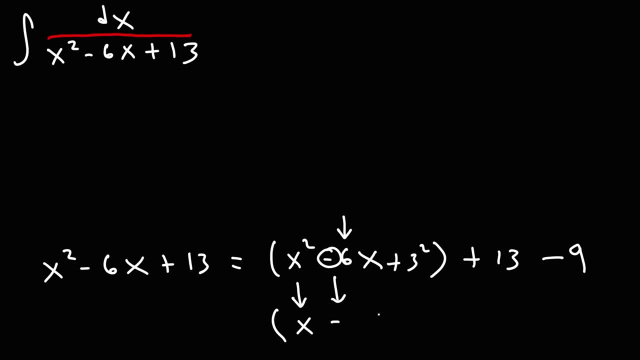 going to be x, whatever. this sign is minus. and then what we see here: 3 squared. That's a quick and simple way to factor a perfect square trinomial. Here we have 13 minus 9, which is 4.. 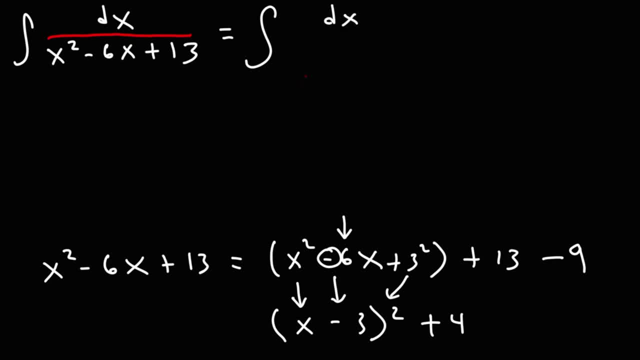 So this is going to be dx, or the integral of dx, over x minus 3, squared plus 4.. So notice the form that we have it in. We almost have it in this form, But we're not quite there yet. What we're going to do is we're going to make u equal to x minus 3.. 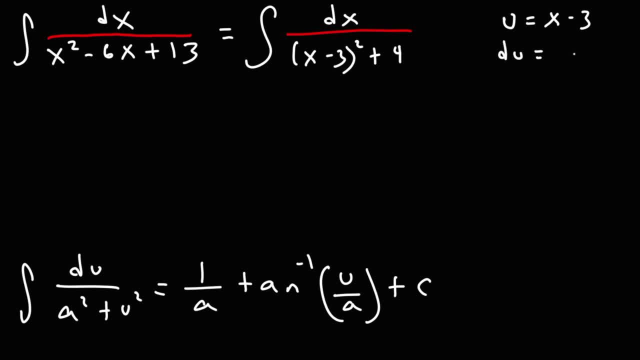 By doing that, du is going to be the derivative of x minus 3,, which is 1.. The derivative of x is 1, but 1dx, So du is equal to dx. So we can replace x minus 3 with u. 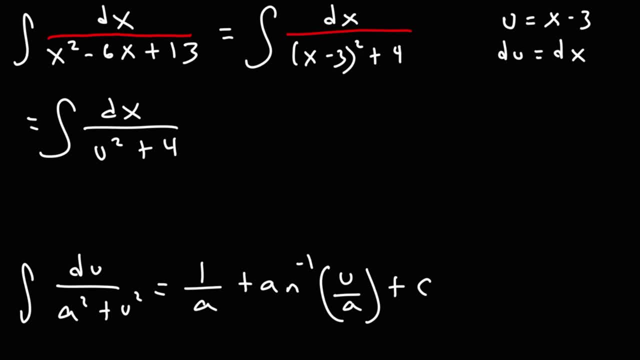 And we're going to have plus 4.. So u squared over 4.. Therefore, we can see that a squared is equal to 4.. If a squared is equal to 4, that means a is equal to 2.. So now we could use this formula: replace an a with 2, and we're going to get 1 over 2. 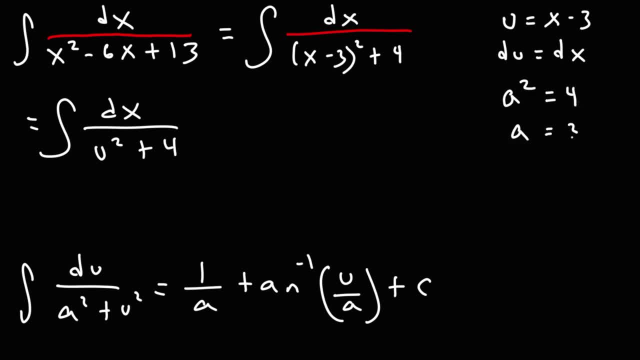 If a squared is equal to 4,, that means a is equal to 2.. So now we could use this formula: replace an a with 2,, And we're going to get 1 over 2, arc tangent u over 2, plus c. 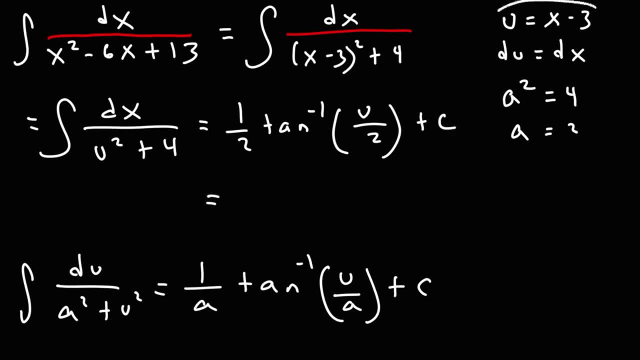 Now the last thing we need to do is get the gi. So this is the深 and this is the subtraction fromют. and then, by subtracting short, squared turns into feet, is: replace u with x minus 3.. So we can leave our final answer as 1 over 2, our 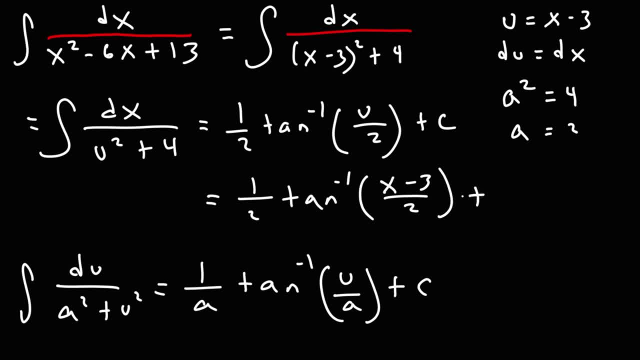 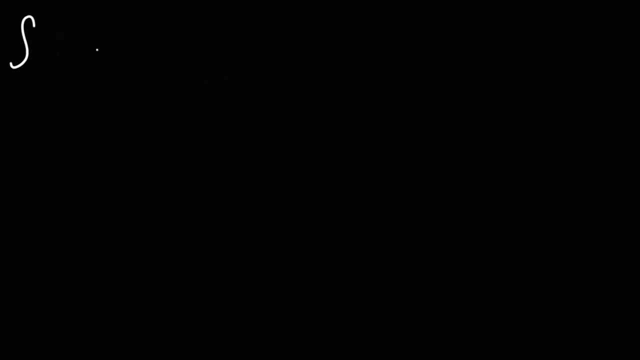 tangent x minus 3 over 2 plus c. So that's how we can integrate this indefinite integral: by completing the square and, of course, using the integration formulas for the inverse trig functions. Now let's work on another problem. Feel free to pause the video if you want to try it. So this problem is going to be. 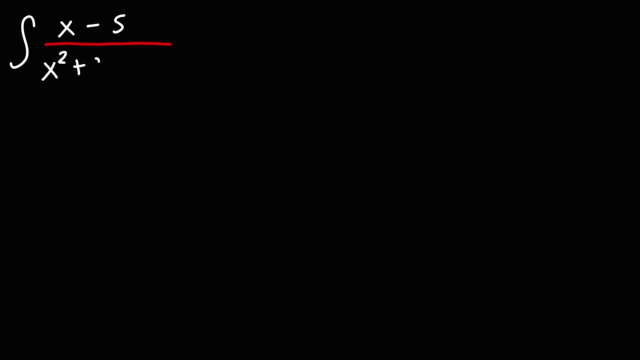 somewhat similar to the last problem, but it's going to be a little bit harder. By the way, for those of you who are looking for more example problems on integration and the various techniques of integration, feel free to check out the links in the description section below. I'm going to. 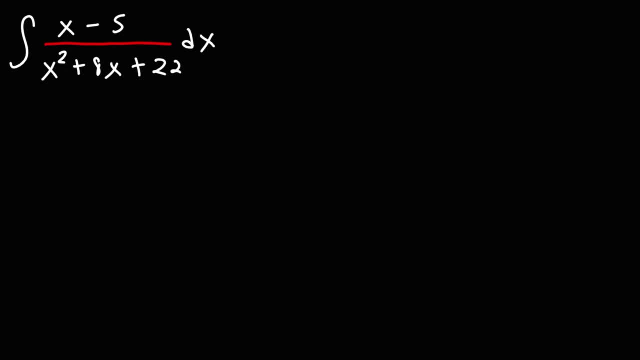 be posting more content in that area. So we could see how this problem is similar to the last one. The only difference is, instead of being, instead of a 1 on top, we have x minus 5.. So, just like before, we're going to complete the square, 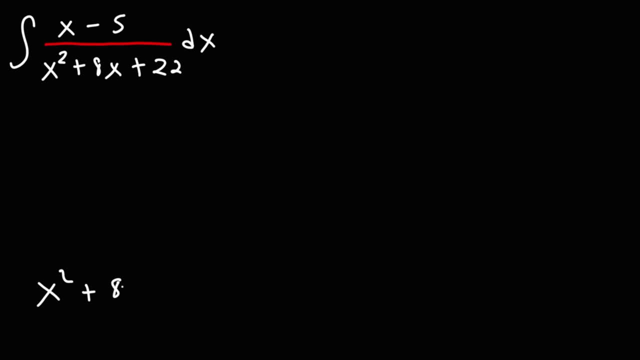 So we have x squared plus 8x plus 22. And that's going to be x squared plus 8x- Let's leave a space- and then plus 22.. So I'm going to take half of 8, which is 4,. 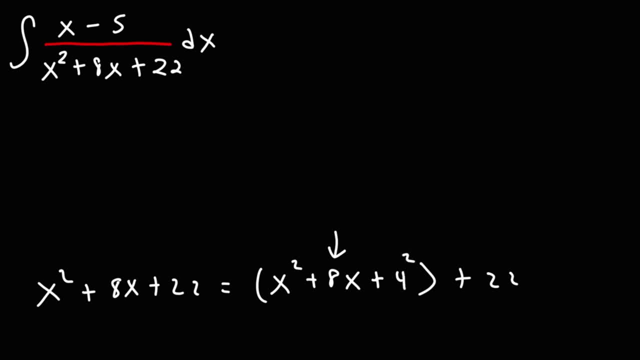 and then I'm going to square it. So 4 squared is 16.. Because I've added 16, I need to take away 16 here. So to factor it, it's going to be x, whatever that sign is plus. and then what we see here: 4 with the squared on. 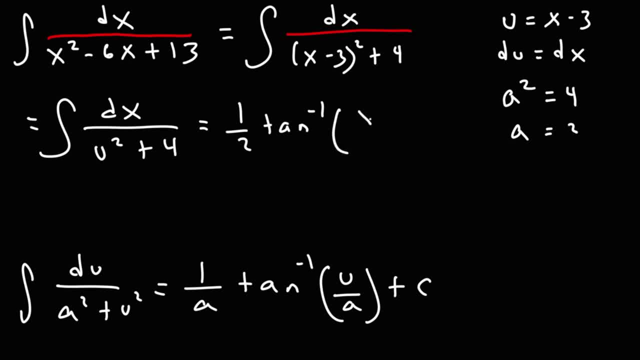 arctangent u over 2 plus c. Now the last thing we need to do is we're going to have u over 2 plus c, So the last thing we need to do is replace u with x minus 3.. So we can leave our final answer as 1 over 2. 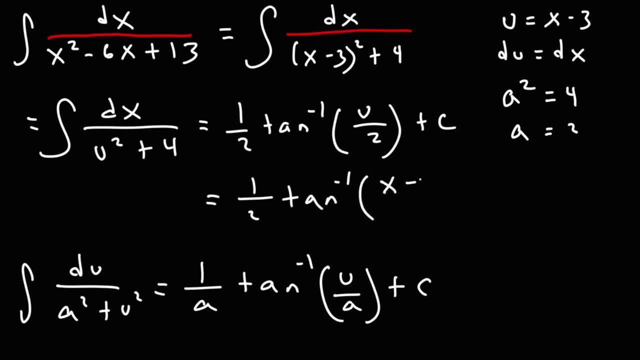 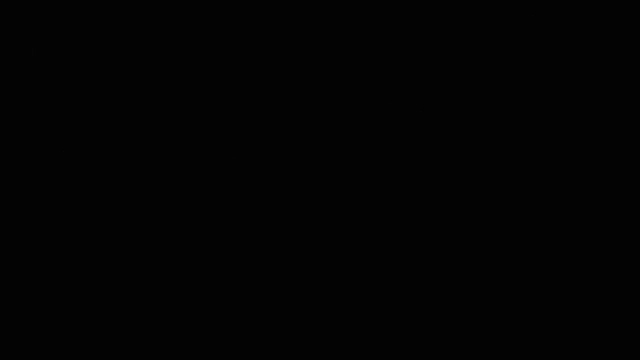 arctangent x minus 3 over 2 plus c. So that's how we can integrate this indefinite integral: by completing the square And, of course, using the integration formulas for the inverse trig functions. Now let's work on another problem. Feel free to pause the video if you want to try it. 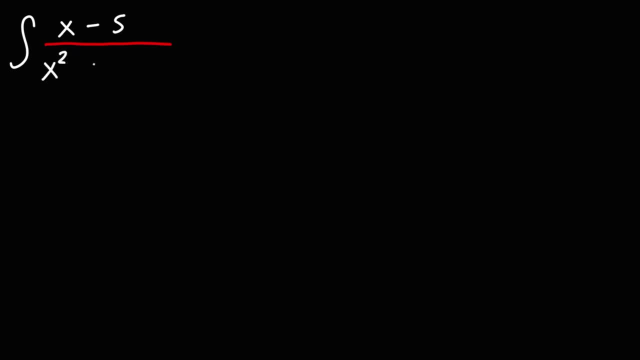 So this problem is going to be somewhat similar to the last problem, but it's going to be a little bit harder. By the way, for those of you who are looking for more example problems on integration and the various techniques of integration, feel free to check out the links in the description section below. 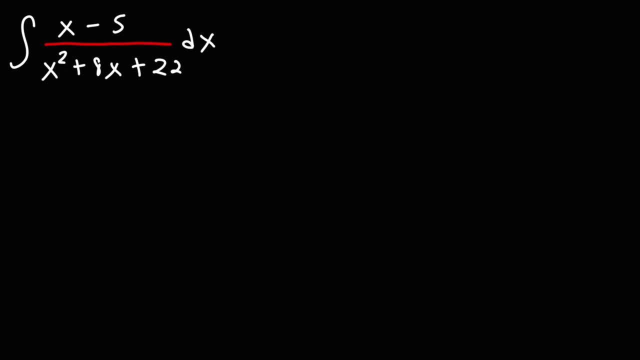 I'm going to be posting more content in that area, So we could see how this problem is similar to the last one. The only difference is, instead of a 1 on top, we have x minus 5.. So, just like before, we're going to complete the square. 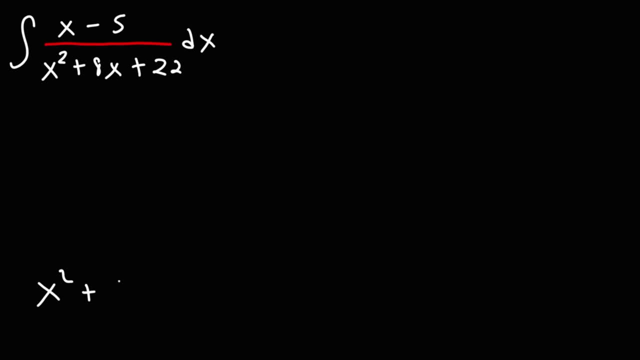 So we have x squared plus 8x plus 22. And that's going to be x squared plus 8x- Let's leave a space- and then plus 22.. So I'm going to take half of 8, which is 4, and then I'm going to square it. 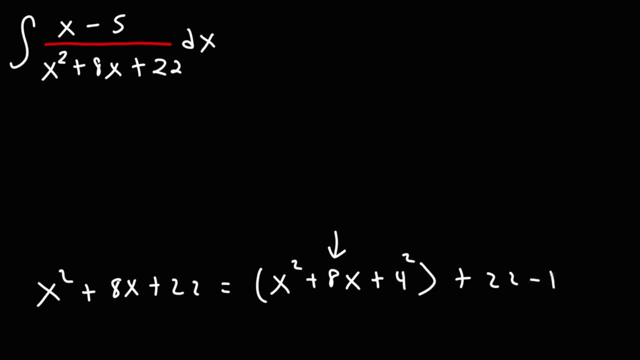 So 4 squared is 16.. Because I've added 16, I need to take away 16 here. So to factor it, it's going to be x plus whatever that sign is plus, and then what we see here. 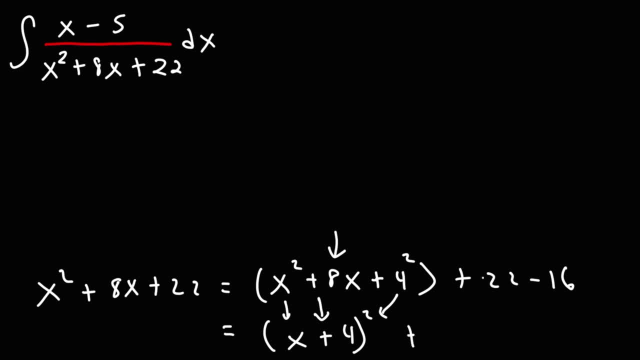 4 with a squared on the outside of the parentheses, And 22 minus 16 is 6.. So we can rewrite this as the integral of x minus 5 over x plus 4, squared plus 6, and then dx. So now let's do some. 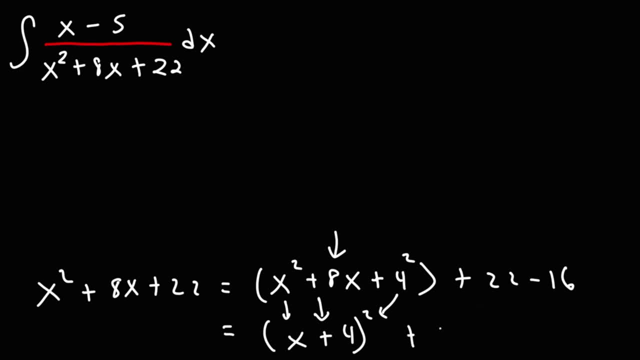 the outside of the parentheses, And 22 minus 16 is 6.. So we can rewrite this as the integral of x minus 5 over x plus 4, squared plus 6 and then dx. So now let's do some use of this. 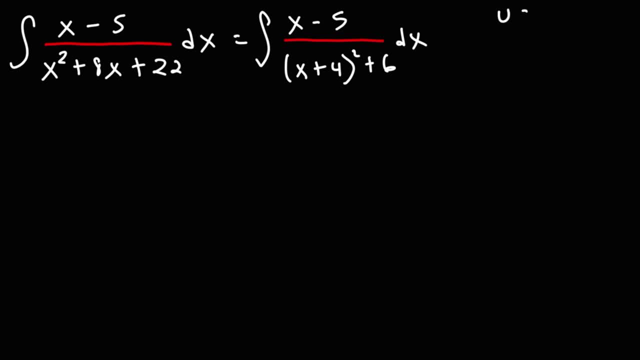 Substitution. So we're going to make u equal to x plus 4.. Therefore, du is going to be equal to dx. Now we can see that we have the u squared plus a squared situation going on here. So this is going to be similar to the arctangent problem. I mean, when we integrate it, we're 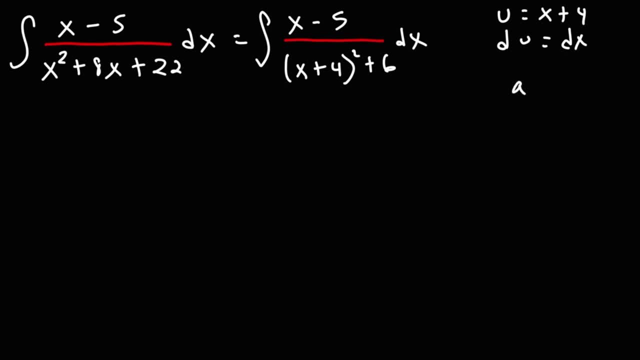 going to get arctangent. So we know that a squared is equal to 6, which means a is going to be equal to the square root of 6.. Now, because we have an x minus 5 here, I need to change the x into a u variable. So in this, 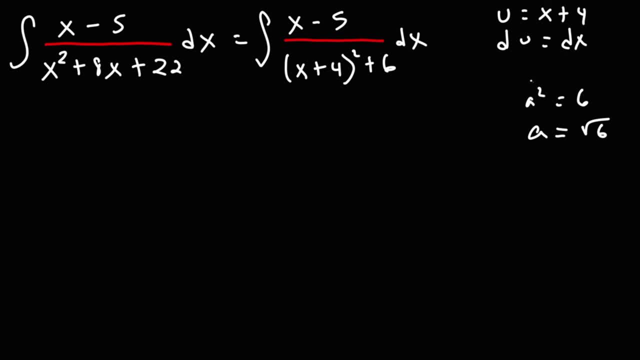 expression I'm going to solve for x, Subtracting both sides by 4, I get that x is equal to u minus 4.. So now I'm going to replace x with u minus 4.. So we have u minus 4 and then minus that 5.. 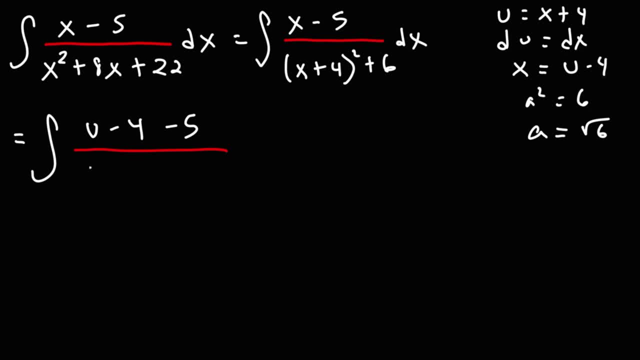 And now I'm going to replace x plus 4 with u, So this is going to be u squared plus 6, and then dx can be replaced with du. So now we have the integral of u minus 9 over u squared plus six, du. Now what we want to do is we want to break up this integral into two. 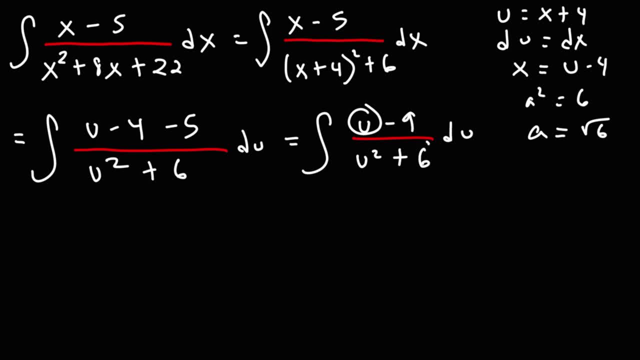 separate integrals. So I'm going to have u divided by the denominator and then separately negative nine divided by the denominator. So the first integral is going to be u over u squared plus six du, And the second one, I'm going to factor out the negative nine, So it's going to be minus nine. 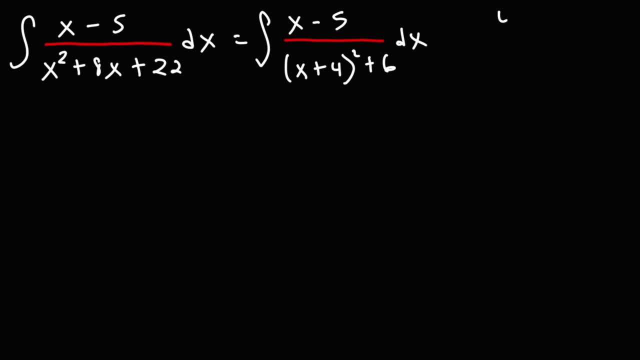 Let's do some u substitution, So we're going to make u equal to x plus 4.. Therefore, du is going to be equal to dx. Now we can see that we have the u squared plus a squared situation going on here, So this is going to be similar to the arctangent problem. 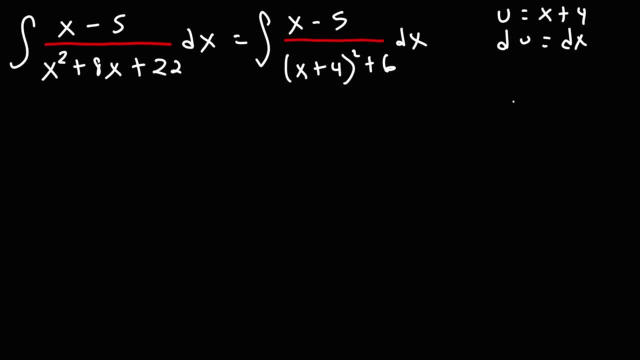 I mean, when we integrate it, we're going to get arctangent. So we know that a squared is equal to 6, which means a is going to be equal to the square root of 6.. Now, because we have an x minus 5 here, I need to change the x into a u variable. 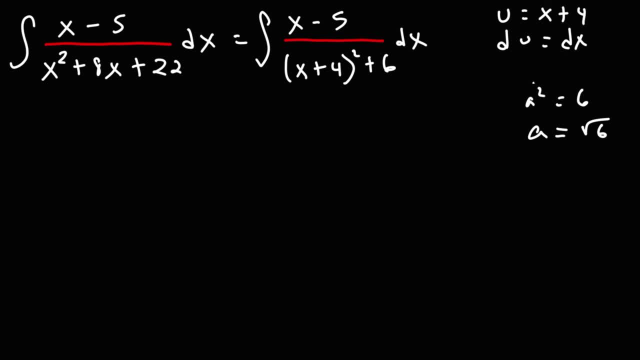 So in this expression I'm going to solve for x, Subtracting both sides by 4, I get that x is equal to u minus 4.. So now I'm going to replace x with u minus 4.. So we have u minus 4 and then minus that 5.. 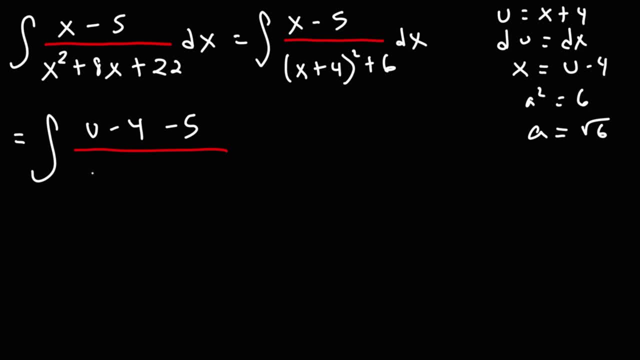 And now I'm going to replace x plus 4 with u, So this is going to be u squared plus 6.. And then dx can be replaced with du, So now we have the integral of u minus 9.. Over u squared plus 6 du. 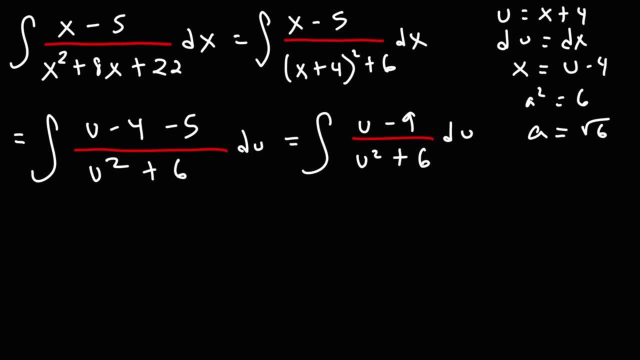 Now what we want to do is we want to break up this integral into two separate integrals. So I'm going to have u divided by the denominator And then separately negative 9 divided by the denominator. So the first integral is going to be u over u squared plus 6 du. 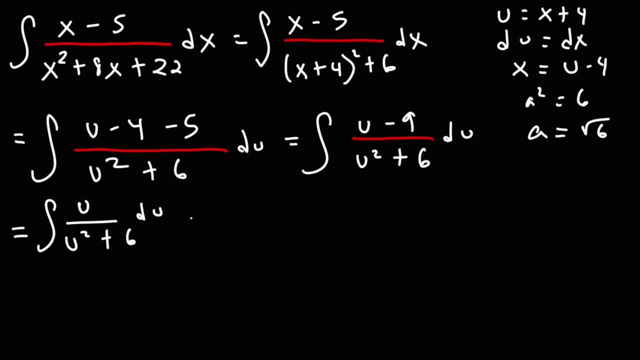 And the second one, I'm going to factor out the negative 9.. So it's going to be minus 9, integral du over u squared plus 6.. Notice, this integral doesn't have anything in the numerator besides du. So that's going to be our arctangent answer. 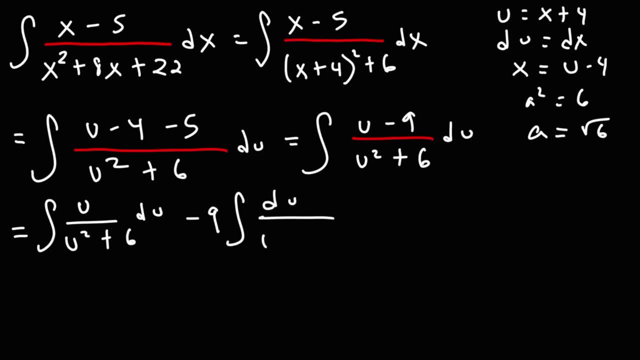 integral du over u squared plus six. Notice this integral doesn't have anything in the numerator besides du. So that's going to be our arctangent answer. This is something else. Notice that the derivative of u squared will give us two u, which can cancel out the u. 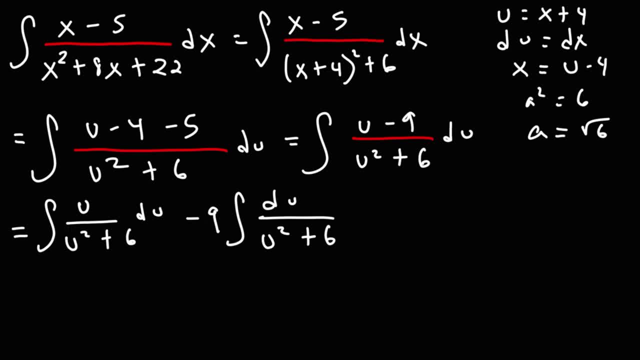 So for that we need to use u substitution. But since we have u already, we'll use a different variable: w substitution or z substitution- It could be any variable you want. Let's use z. So I'm going to make z equal to u squared plus six dz. The derivative of that is going to be: 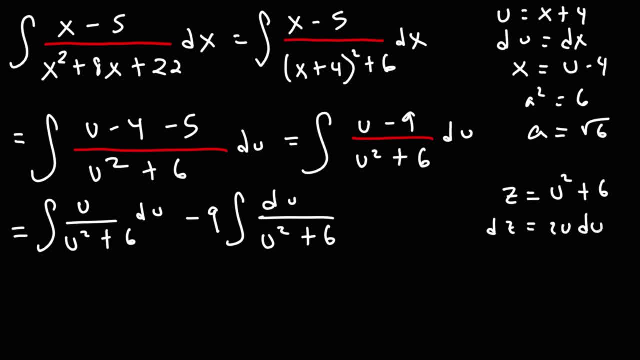 the derivative of u squared, which is two u, and then times du, So solving for du. I'm going to get the derivative of u squared plus six du, So I'm going to get the derivative of u squared plus six du, So I'm going to get dz divided by two. u is equal to du. 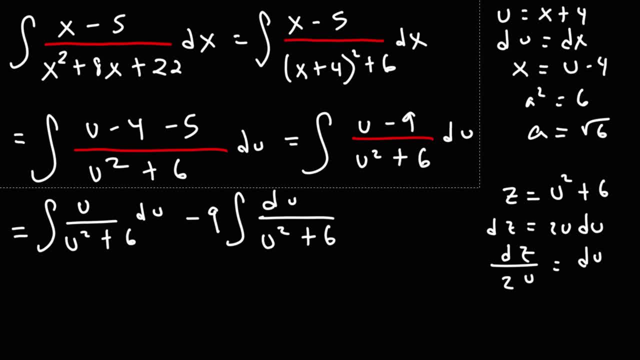 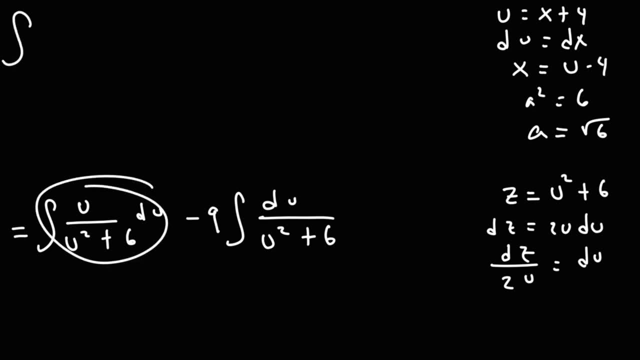 So let's get rid of this in the meantime. So I'm going to focus on evaluating that integral real quick. So the integral of u over u squared plus six, du, that's going to be u divided. by now, u squared plus six. I'm going to replace that with z. 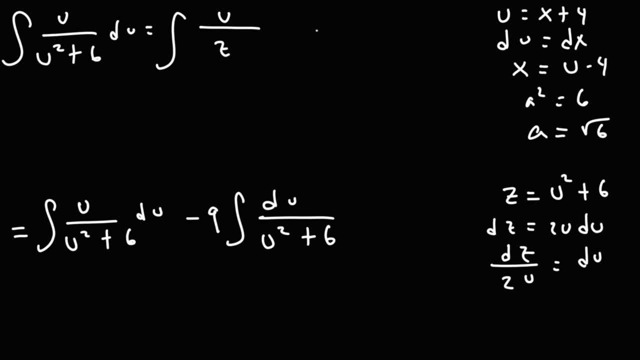 And du. I'm going to replace that with dz over two u So we could cancel out the u variable, The one half. I'm going to move to the front, So I have one half integral, one over z, dz. We know the antiderivative of one over x is ln, x. 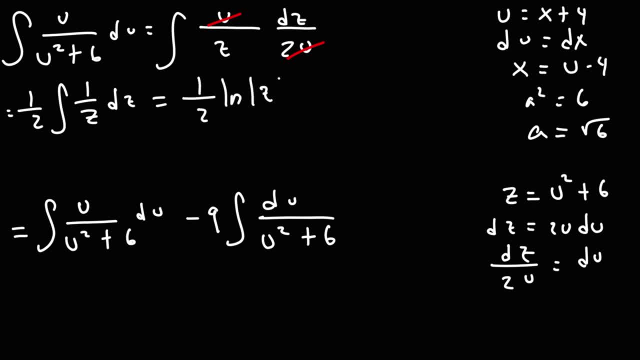 So one over z becomes ln z, And of course we can put plus c. But we could put plus c at the very end of the problem. Now I need to replace z with u squared plus six. Now I no longer need the absolute value, because u squared plus six will always be positive. 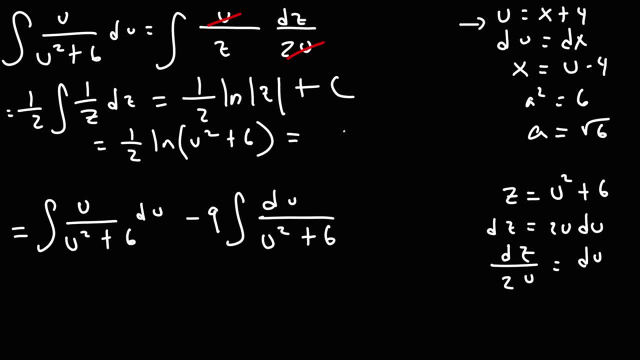 And then, finally, I need to replace u with x plus four. Notice, this is the factored form of the denominator that we had right after when we complete the square. If you were the FOIA of x plus four times x plus four, and then add six to it. 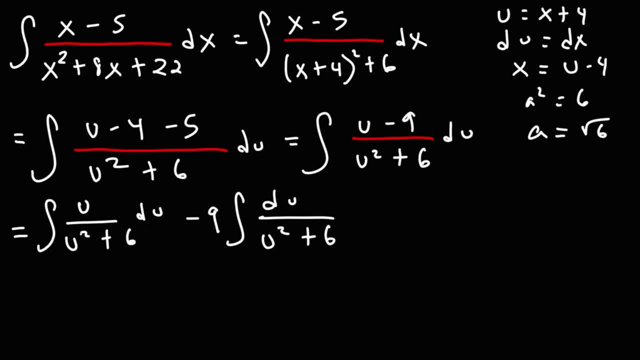 This is something else. Notice that the derivative of u squared will give us 2u, which can cancel out the u. So for that we need to use u substitution. But since we have u already, we'll use a different variable. 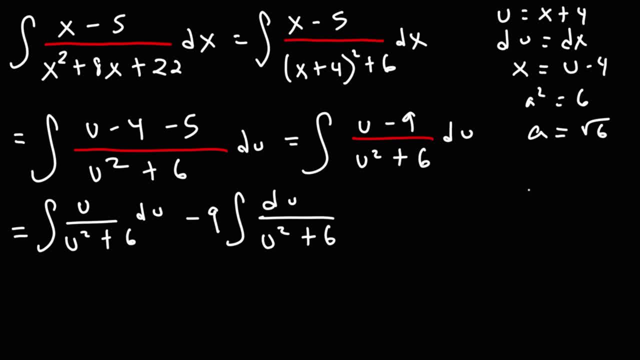 W substitution Or z substitution, It could be any variable you want. Let's use z. So I'm going to make z equal to u squared plus 6. dz, the derivative of that, is going to be the derivative of u squared, which is 2u, and then times du. 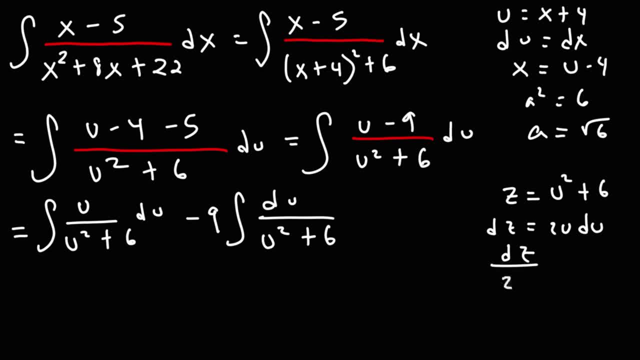 So, solving for du, I'm going to get dz divided by 2u. So I'm going to get dz divided by 2u. 2u is equal to du, So let's get rid of this in the meantime. So I'm going to focus on evaluating that integral real quick. 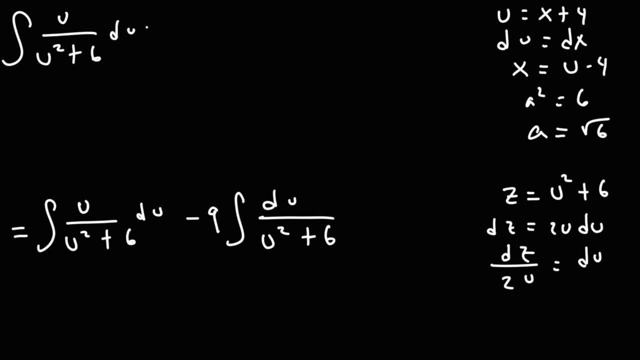 So the integral of u over u squared plus 6, du, That's going to be u divided by u squared plus 6, I'm going to replace that with z And du. I'm going to replace that with dz over 2u. 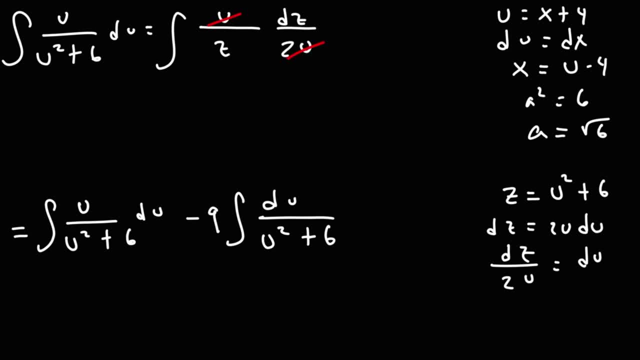 So we could cancel out the u variable, The 1 half. I'm going to move to the front. So I have 1 half. integral 1 over z dz. We know the antiderivative of 1 over x is ln, x. 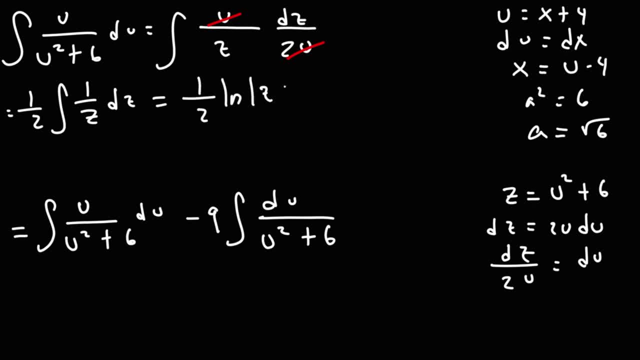 So 1 over z becomes ln, z And of course plus c. But we could put plus c at the very end of the problem. Now I need to replace z with u squared plus 6. Now I no longer need the absolute value. 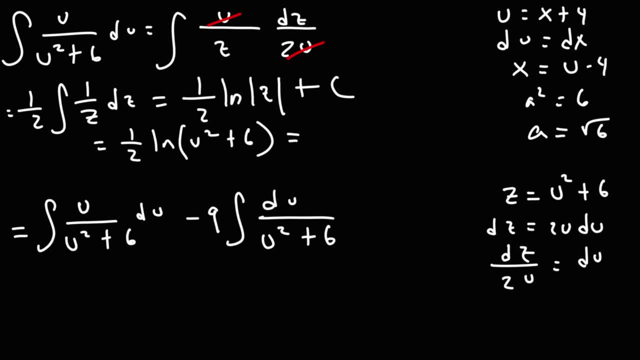 because u squared plus 6, will always be positive. And then, finally, I need to replace u with x plus 4.. Notice, this is the factored form of the denominator that we had right after when we complete the square, If you were to FOIL x plus 4 times x plus 4 and then add 6 to it. 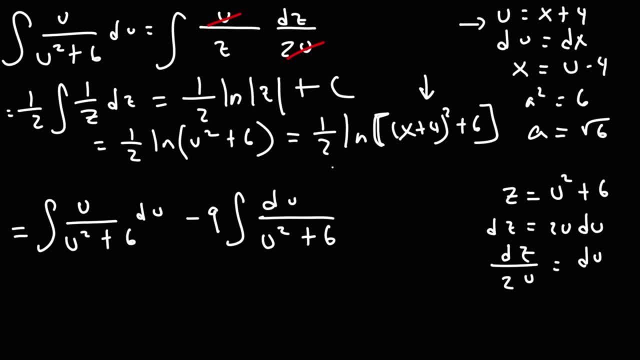 you would get the denominator of the original problem, which I could put that answer here. That's going to be 1 half ln x squared plus 8x. You know, 4x plus 4x will give us 8x. 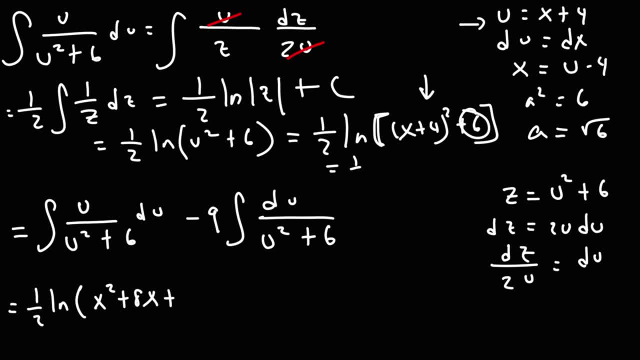 And then 4 times 4 will give us 16 plus 6. That will give us 22.. So that's the polynomial that we had in the beginning in the denominator of the integral. So that covers this integral. Now we've got to focus on this one. 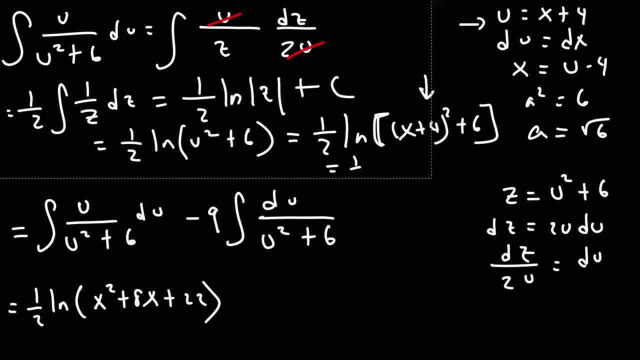 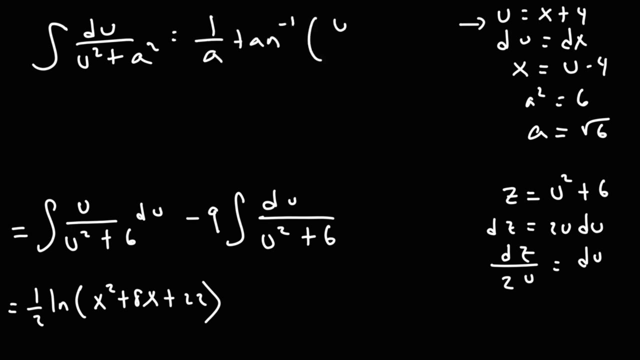 So this is going to be. We know the integral of du over u squared plus a. squared, It's 1 over a arctangent, u over a plus c. Now we already have it in the appropriate form And we know that a is equal to the square root of 6.. 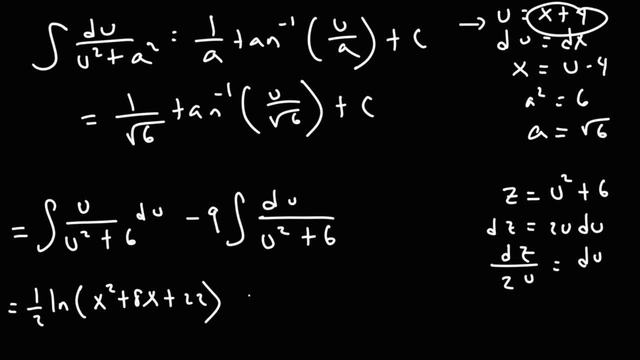 And we know that u is x plus 4.. So this is going to become- And we can't forget about the negative 9.. So it's negative 9.. If you multiply these two, this becomes negative 9 over the square root of 6.. 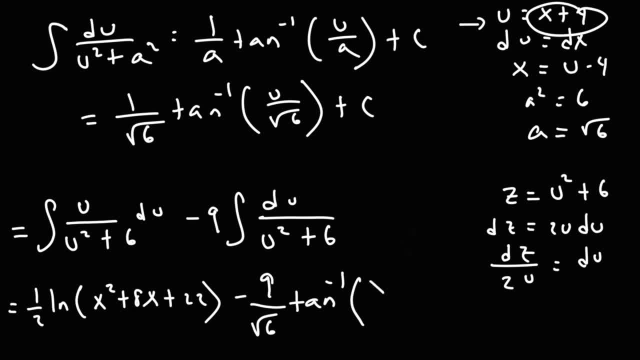 And then times arctangent, replacing u with x plus 4, we have x plus 4 over the square root of 6 plus c. So that, right, there is the final answer for this problem, Unless, of course, you want to rationalize. 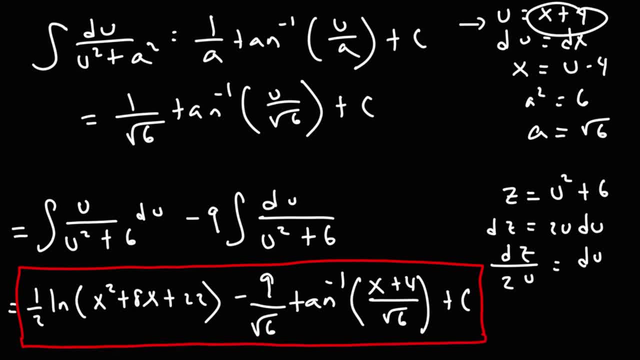 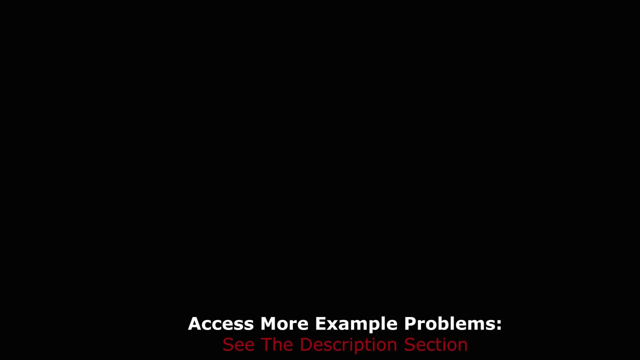 the square root of 6 on the denominator of those fractions. But if you get to this point, you have the right answer. Most professors- hopefully they'll accept it like this. Now let's work on a different problem. What is the integral of 1 over the square root? 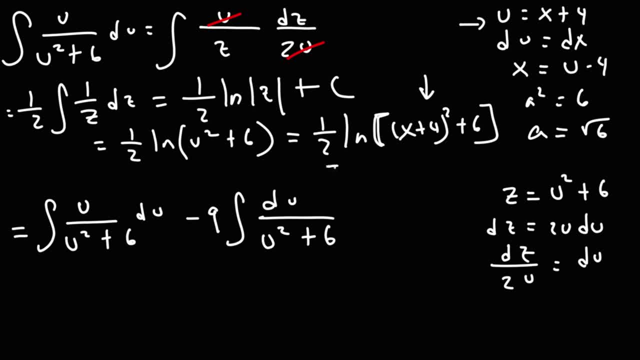 you would get the denominator of the original problem, Which I could put that answer here. That's going to be one half ln x squared plus 8x minus 1. You know, 4x plus 4x will give us 8x, and then 4 times 4 will give us 16, plus 6, that will give us 22.. 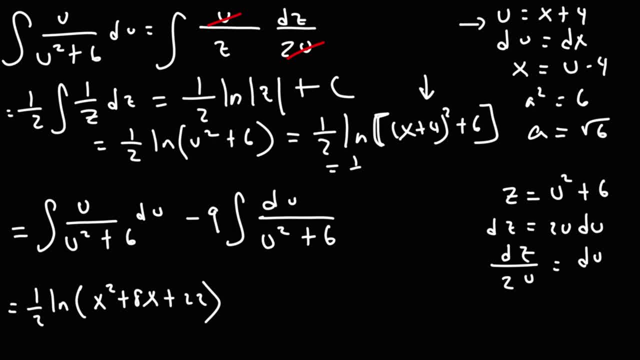 So that's the polynomial that we had in the beginning in the denominator of the integral. So that covers this integral. Now we've got to focus on this one. So this is going to be, we know, the integral of du over u squared plus a squared. 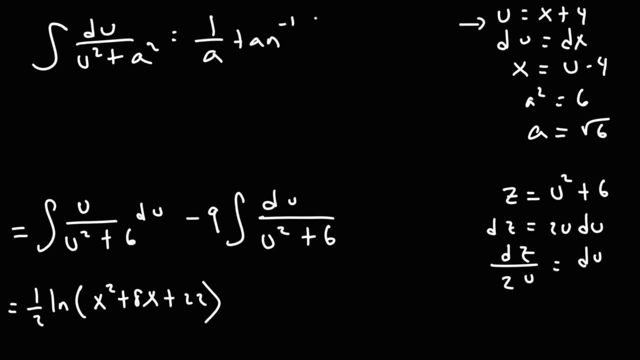 It's 1 over a arctangent, u over a plus c. Now we already have it in the appropriate form And we know that a is equal to the square root of 6. And we know that u is x plus 4.. 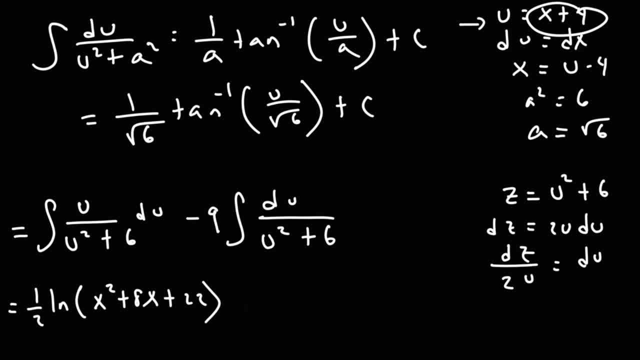 So this is going to become, and we can't forget about the negative 9.. So it's negative 9, if you multiply these two, this becomes negative 9 over the square root of 6.. And then times arctangent, replacing u with x plus 4, we have 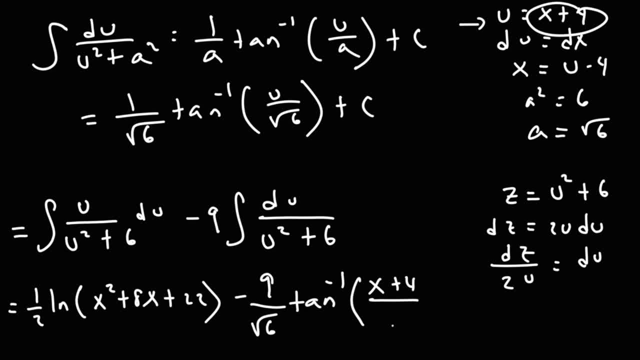 x plus 4 over the square root of 6 plus c. So that, right, there is the final answer for this problem, Unless, of course, you want to rationalize the square root of 6 on the denominator of those fractions. But if you get to this point, you have the right answer. 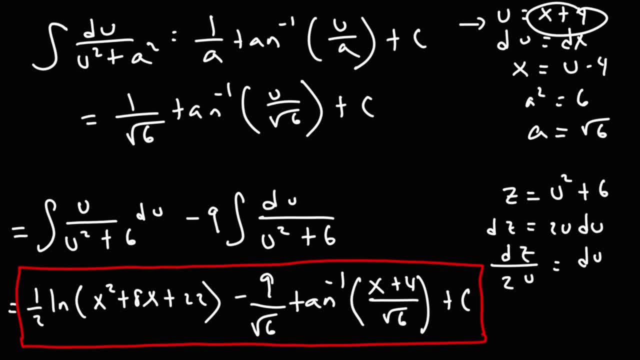 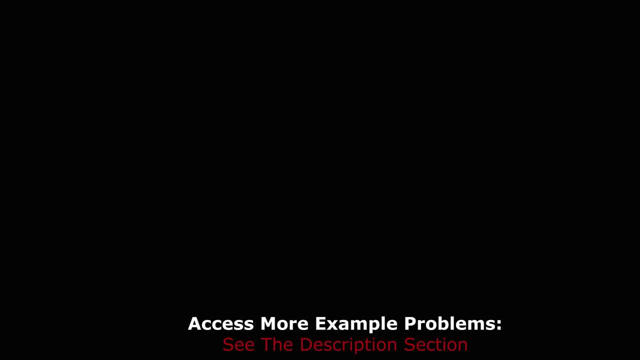 Most professors. hopefully they'll accept it like this. Now let's work on a different problem. What is the integral of 1 over the square root of negative x squared minus 6x dx? Feel free to pause the video if you want to try that. 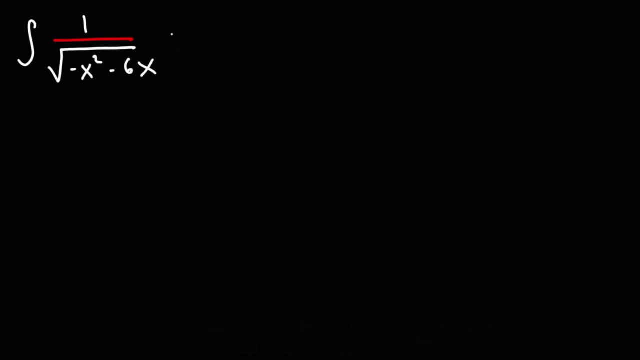 of negative x squared minus 6x dx. Feel free to pause the video if you want to try that Now, because we have a square root in the bottom. we're not dealing with arctangent, So is this arcsecant or arcsine? 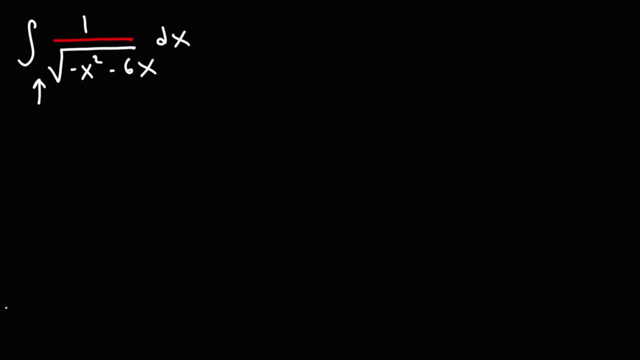 Notice that we don't have another x variable outside of the radical, So this is likely to be arcsine, which has this form: The integral of du over the square root of a squared minus u squared is equal to arcsine: u over a plus c. 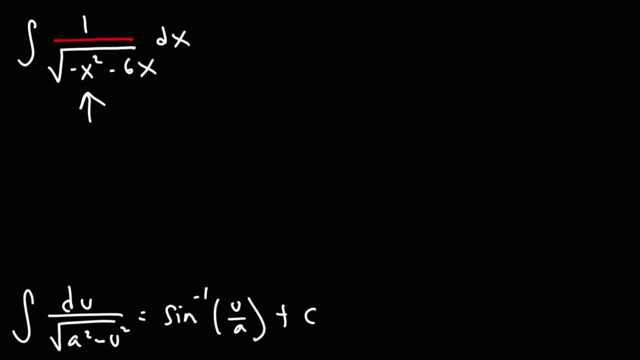 So negative u squared. that looks similar to negative x squared. We don't see the a squared yet, but we could introduce a squared if we complete the square. So let's go ahead and do that. So we have negative x squared minus 6x. 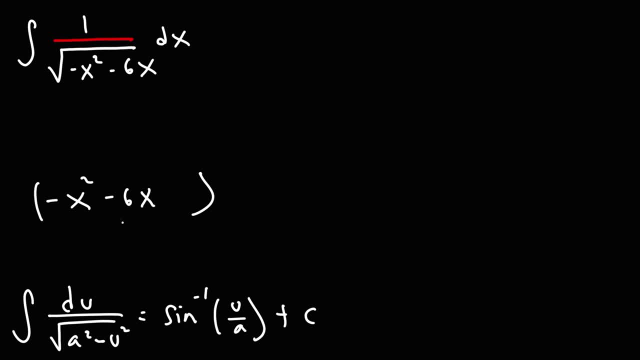 Now, before we complete the square, we need to factor out a negative 1.. So we're going to have negative 1 x squared plus 6x. I'm going to leave a space And now let's complete the square. So half of 6 is 3,. 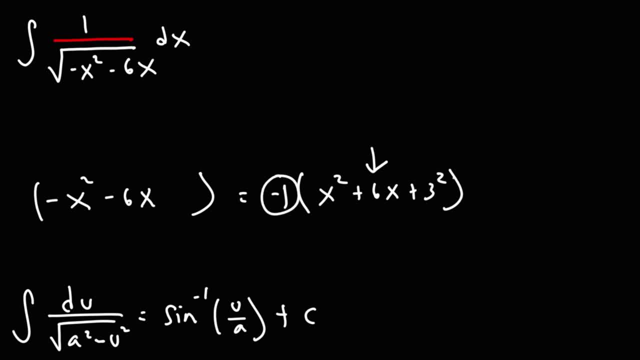 so I'm going to add 3 squared. So notice that I've added not positive 9, but negative 9 because of the negative sign in front. So because I've added negative 9 to this expression in order to maintain the value. 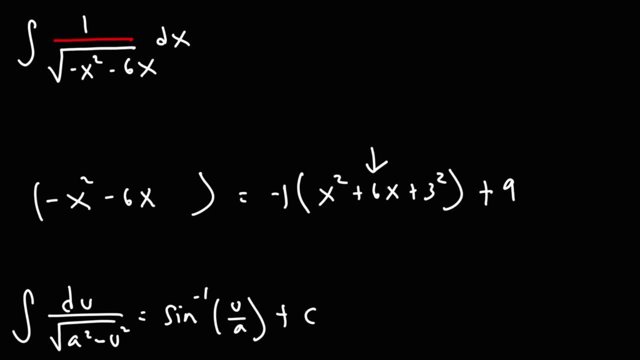 I need to add positive 9 to it. So now this becomes negative 1. When we factor it, it's going to be x plus 3 squared, and then plus 9.. Now I'm going to rewrite this, because this is negative. 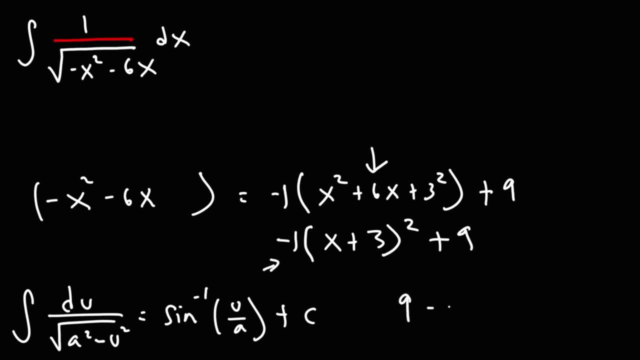 I like to put the positive term in front, So I'm going to write this as negative. I mean 9 minus x plus 3 squared. So now we can see it's in the form a squared minus u squared where a squared is negative. 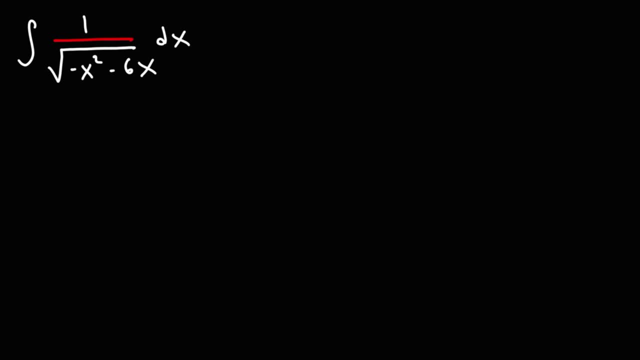 Now, because we have a square root of negative x squared, we have a square root of 6x dx, We have a square root in the bottom. We're not dealing with arctangent, So is this arc secant or arc sine? 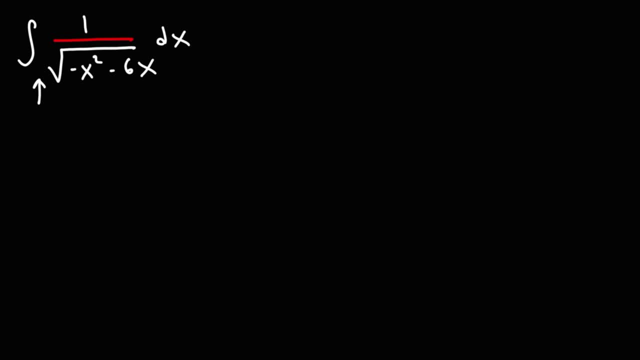 Notice that we don't have another x variable outside of the radical, So this is likely to be arc sine, which has this form: The integral of du over the square root of a squared minus u squared is equal to arc sine u over a plus 6x. 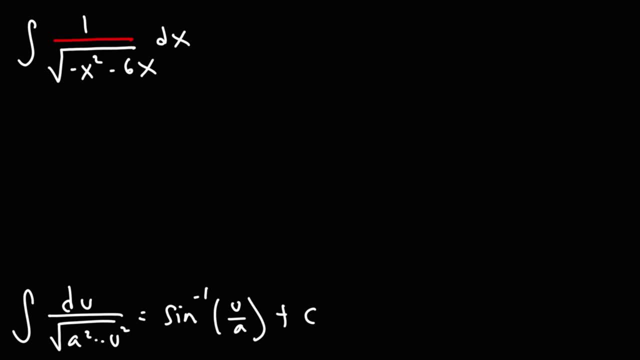 That's the influence of of x squared. So negative u squared that looks similar to negative x squared. We don't see the a squared yet, but we could introduce a squared if we complete the square. So let's go ahead and do that. 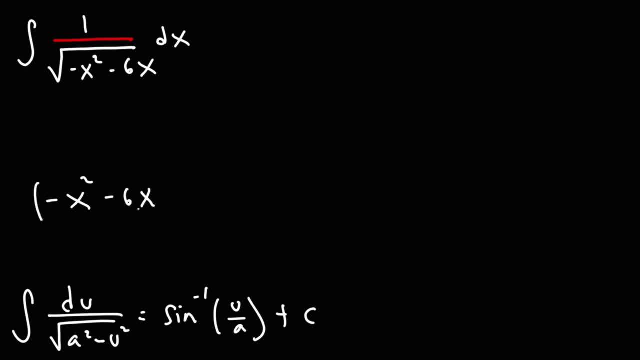 So we have negative x squared minus 6x. Now, before we complete the square, we need to factor out a negative 1.. So we're going to have negative 1x squared plus 7x- 6x. I'm going to leave a space, and now let's complete the square. So half of 6 is 3, so I'm. 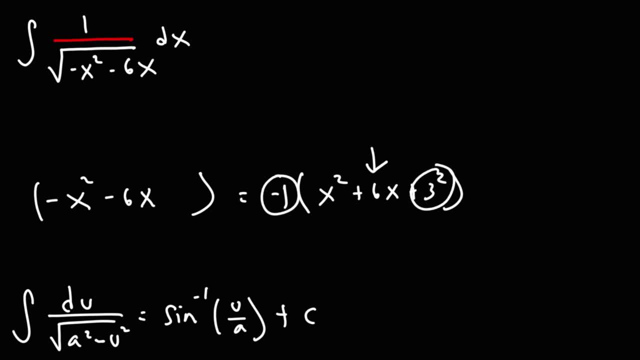 going to add 3 squared. So notice that I've added not positive 9, but negative 9 because of the negative sign in front. So because I've added negative 9 to this expression, in order to maintain the value I need to add positive 9 to it. So now this becomes negative 1. When we factor 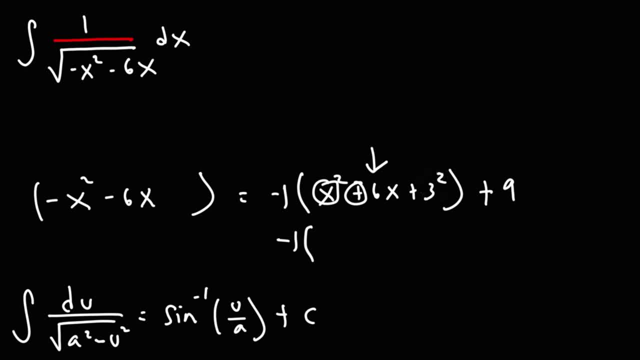 it. it's going to be x plus 3 squared and then plus 9.. Now I'm going to rewrite this because this is negative. I like to put the positive term in front, So I'm going to write this as negative. I mean 9 minus x plus 3 squared. So now we can see it's in the form a squared minus u squared. 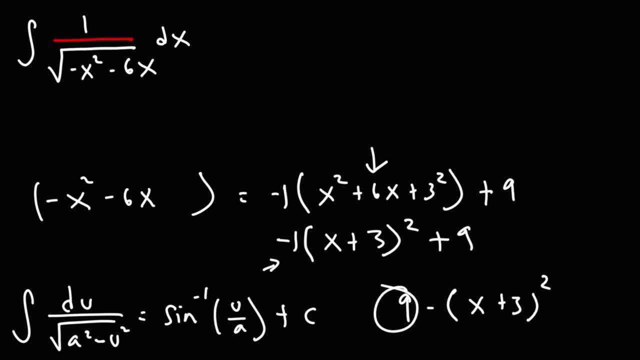 where a squared is 9, u squared is x minus x 3 squared. So let's rewrite this as the integral of dx divided by the square root of 9 minus x plus 3 squared. So now we're going to make u equal to x plus 3.. Therefore, du is going to be equal. 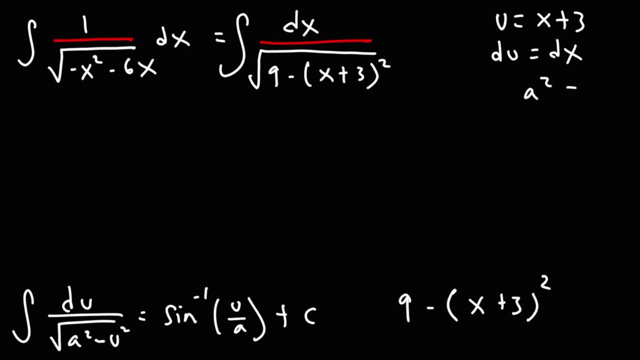 to dx, And we know that a squared is 9, which means a is the square root of 9.. Therefore, a is 3.. So we're going to have the integral of. let's replace dx with du, since they're. 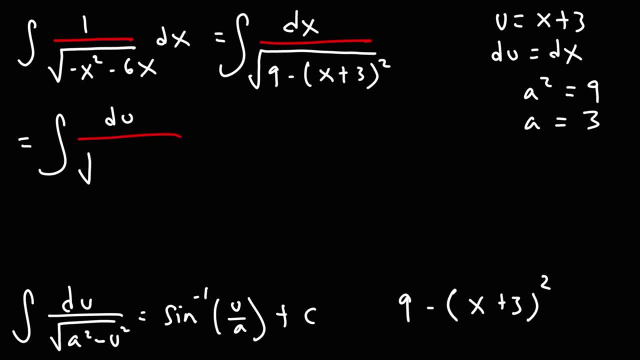 equal to each other, And if you want to, you can replace 9 with 3 squared, And then x plus 3 is u, so this becomes u squared. So now it looks exactly like that. So now we just got to plug in what. 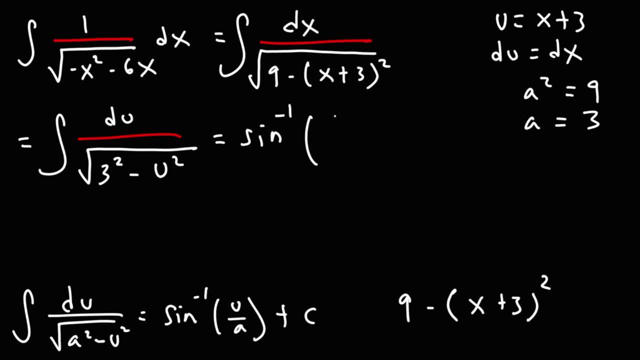 we have. So this becomes arc sine u over a. a is 3, plus c, And then let's replace u with x plus 3.. And so that is the answer. As you can see, this problem wasn't too bad, even though it. 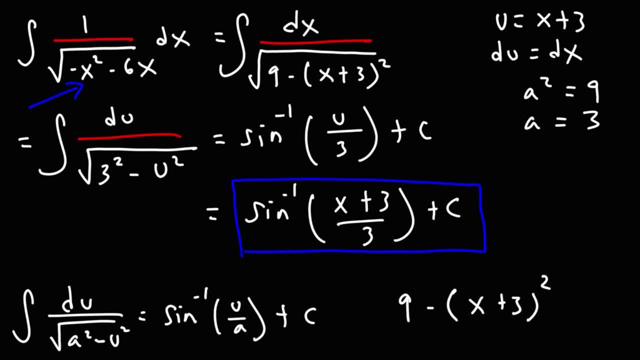 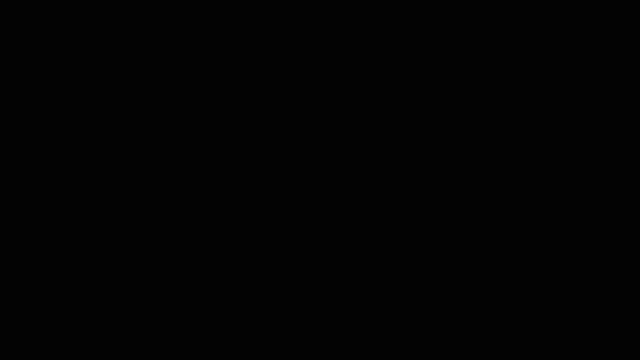 may look difficult with the negative x squared inside of the radical, But now let's move on to our next problem. So feel free to pause the video if you want to try that, Like before. let's go ahead and complete the square. So starting with negative x squared. 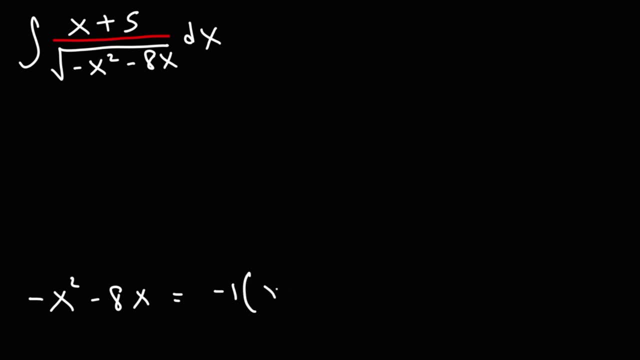 minus 8x. let's begin by factoring out the negative 1.. So this becomes x squared plus 8x. Let's leave a space Now to complete the square. we're going to take half of 8, which 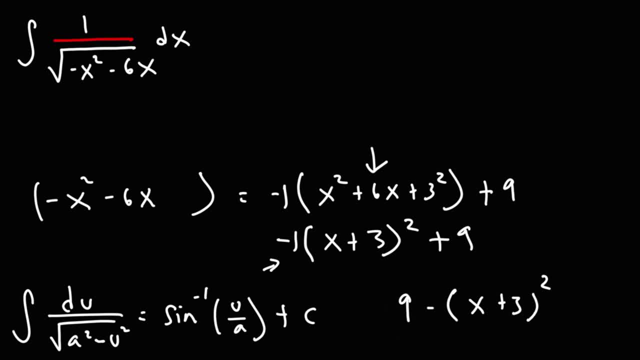 a squared is 9, u squared is x plus 3 squared. So let's rewrite this as the integral of dx divided by the square root of 9 minus x plus 3 squared. So now we're going to make u equal to x plus 3.. 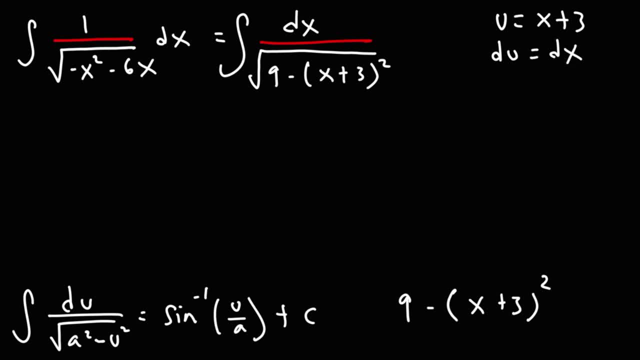 Therefore, du is going to be equal to dx, And we know that a squared is 9,, which means a is the square root of 9, therefore a is 3.. So we're going to have the integral of. let's replace dx with du. 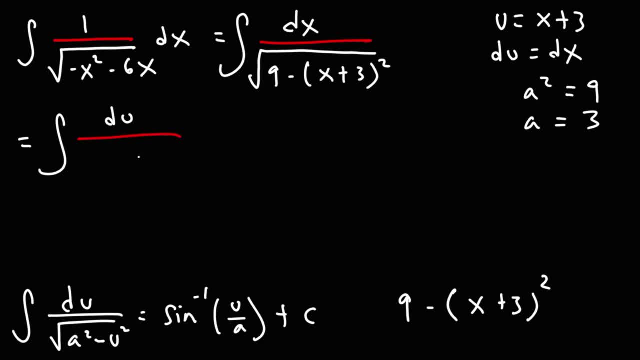 since they're equal to each other. And if you want to, you can replace 9 with 3 squared, And then x plus 3 is u, so this becomes u squared. So now it looks exactly like that. So now we just got to plug in what we have. 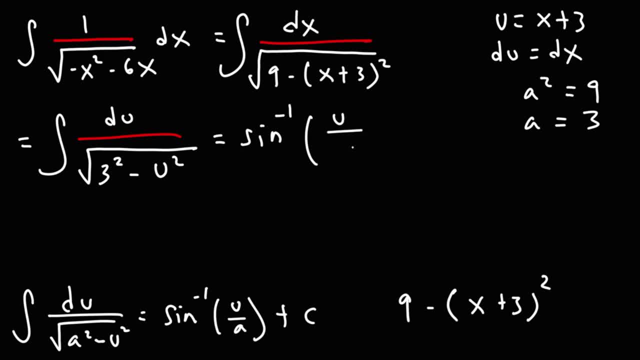 So this becomes: arc sine u over a, a is 3, plus c, And then let's replace u with x plus 3.. And so that is the answer. As you can see, the problem wasn't too bad, even though it may look difficult. 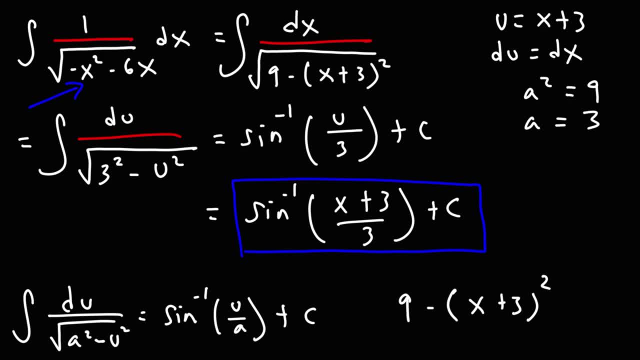 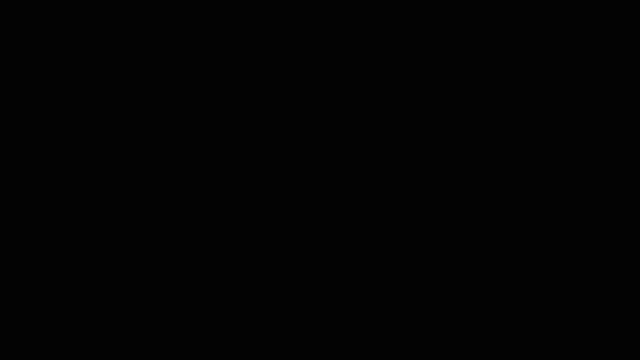 with the negative x squared inside of the radical. But now let's move on to our next problem. So feel free to pause the video if you want to try that, Like before, let's go ahead and complete the square, So starting with negative x squared minus 8x. 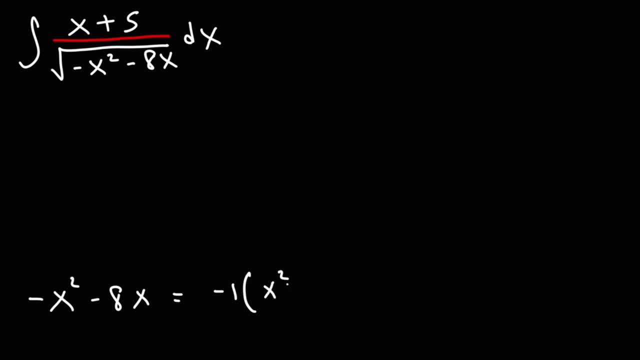 let's begin by factoring out the negative 1.. So this becomes x squared plus 8x. Let's leave a space Now to complete the square. we're going to take half of 8,, which is 4.. So we're going to add plus 4 squared. 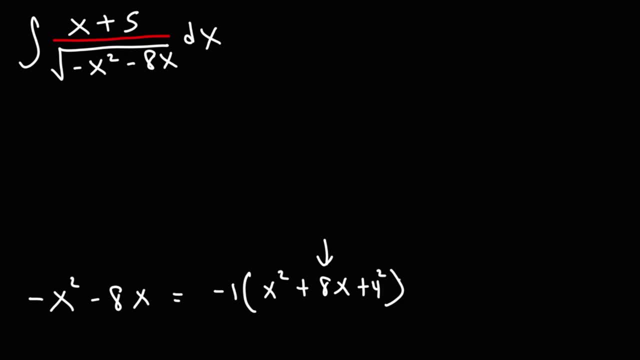 is 4.. So we're going to add plus 4 squared Now, because we added not positive 16, but negative 16, to undo that we need to add positive 16.. So the factor it's going to be x plus 4 squared and then plus 16,, which I'm going to reverse. 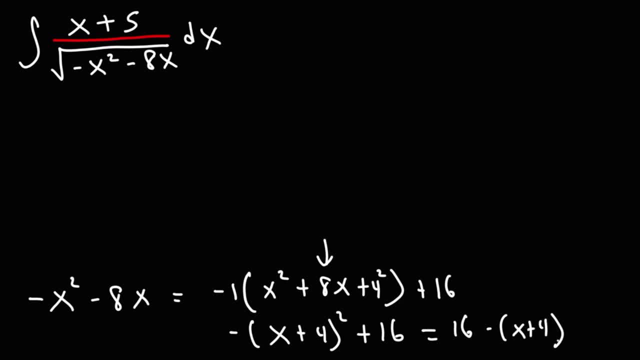 the 2 and write it this way to put it in the appropriate format. So what we have is the integral of x plus 5 over the square root of 16, minus x plus 4 squared dx. So, just like before, we're going to make u equal to x plus 4 squared. 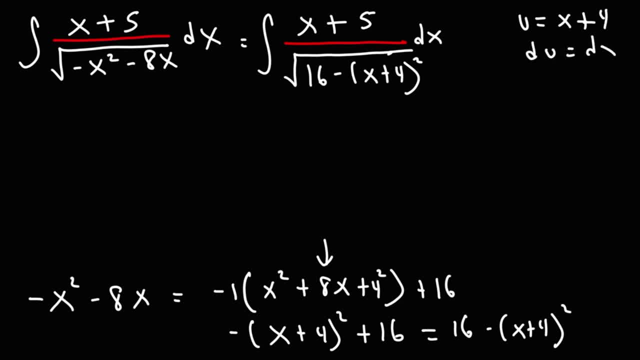 which means du is equal to dx. Now we can see that a squared is 16 and the square root of 16 is 4.. Now notice that we have an x plus 5 on top. So, like the second problem in this video, we're going to solve for x over here, Subtracting both. 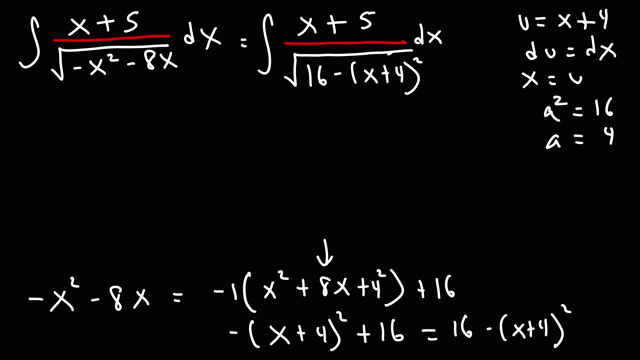 sides by 4, we get that u minus 4 is equal to x. So now let's substitute, Let's replace x with u minus 4.. And then we have a plus 5.. This is divided by the square root. Now, instead of 16, I'm going to write it as 4 squared, So you can see. 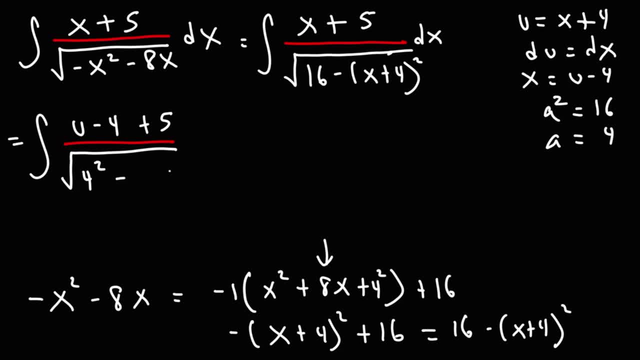 that it will remind you that a is 4.. And x plus 4,. let's replace that with u And dx. we can replace that with du, So this becomes the integral of u. Negative 4 plus 5 is plus 1.. 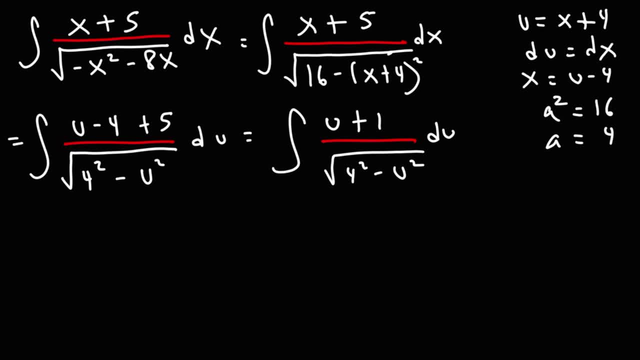 Now, just like the second problem, we're going to break this apart into two integrals. So we're going to have the integral of u divided by the square root of 4 squared minus u squared, And to solve that one we could just use a normal substitution. 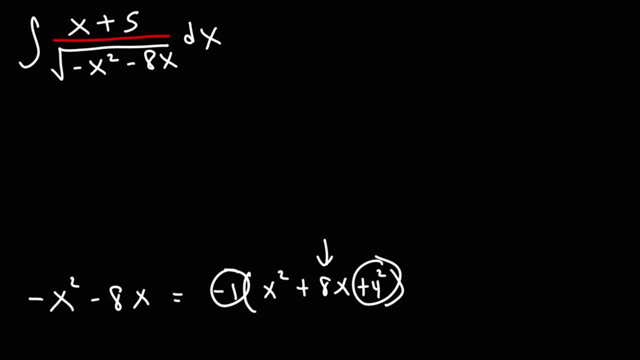 Now, because we added not positive 16, but negative 16, to undo that, we need to add positive 16.. So the factor it's going to be x plus 4 squared and then plus 16,, which I'm going to reverse the 2 and write it this way: 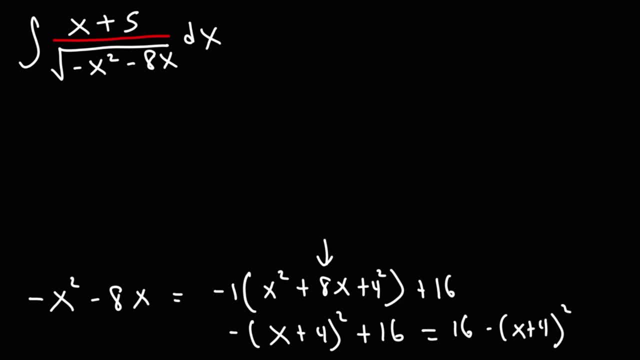 to put it in the appropriate format. So what we have is the integral of x plus 5 over the square root of 16, minus x plus 4 squared dx. So, just like before, we're going to make u equal to x plus 4,. 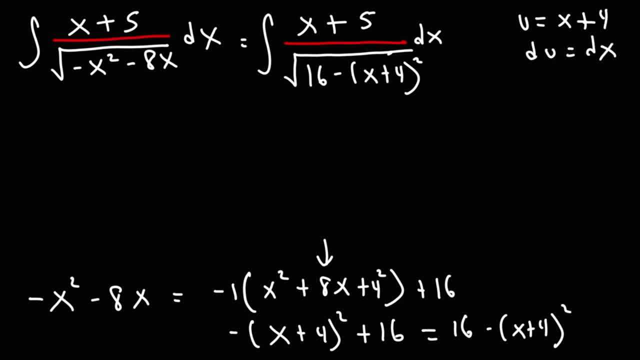 which means du is equal to dx. Now we can see that a squared is 16, and the square root of 16 is 4.. Now notice that we have an x plus 5 on top. So like the second problem in this video, 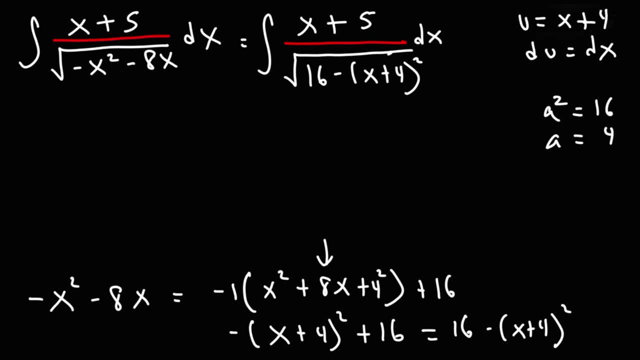 we're going to solve for x over here. Subtracting both sides by 4, we get that u minus 4 is equal to x. So now let's substitute, Let's replace x with u minus 4.. And then we have a plus 5.. 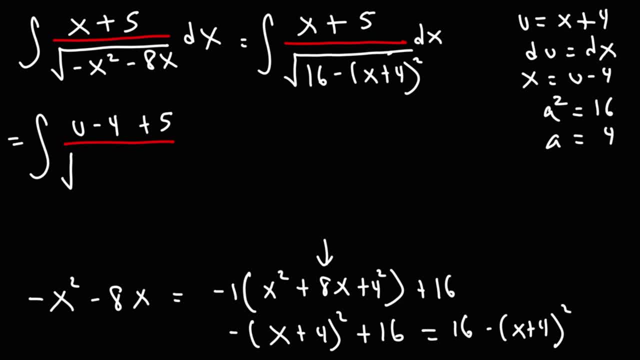 This is divided by the square root. Now, instead of 16,, I'm going to write it as 4 squared, So you can see that. it will remind you that a is 4. And x plus 4, let's replace that with u. 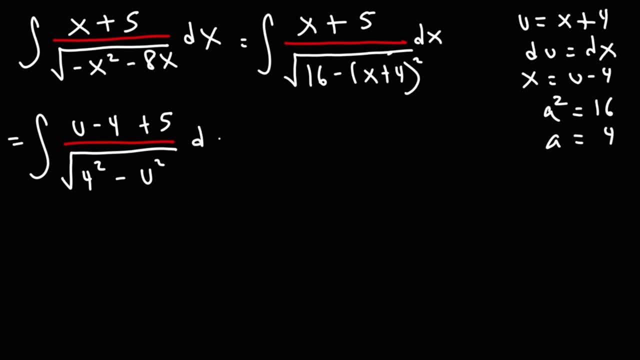 And dx. we can replace that with du, So this becomes the integral of u. negative 4 plus 5 is plus 1.. Now, just like the second problem, we're going to break this apart into two integrals, So we're going to have the integral of u. 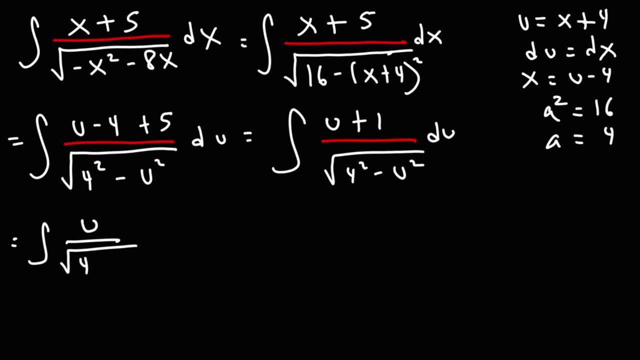 divided by the square root of 4 squared minus u squared. And to solve that one we could just use a normal substitution, u substitution, integration technique, And for this one this is going to be our arc sine formula. So let's go ahead and use u substitution on this. 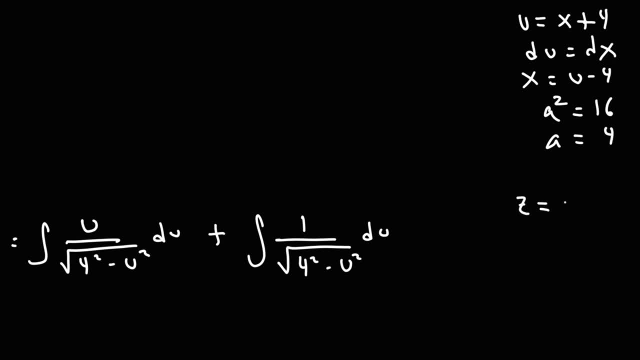 So let's introduce a new variable which we'll call z. So z is going to be 16 minus u squared And dz the derivative of negative u squared, that's negative 2u du. Solving for du, we get dz over negative. 2u is du. 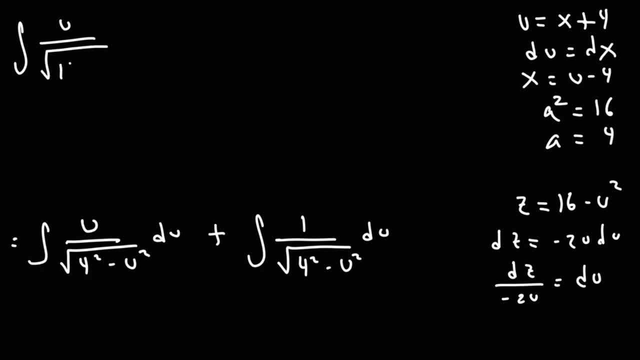 So, focusing on this integral, we have this. So I'm going to keep the u, I'm going to replace 16 minus z squared, I mean 16 minus u squared with z, And du is going to be dz over negative 2u. 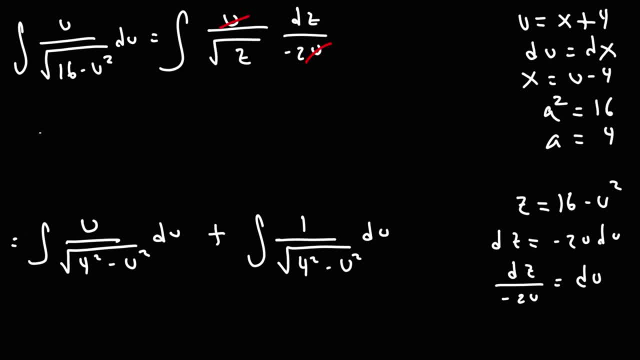 So we could cancel out the u And we can move the negative 1 half to the front. So we have this Now: z- the square root of z is z- to the half, And if we were to move that z to the top of the fraction, 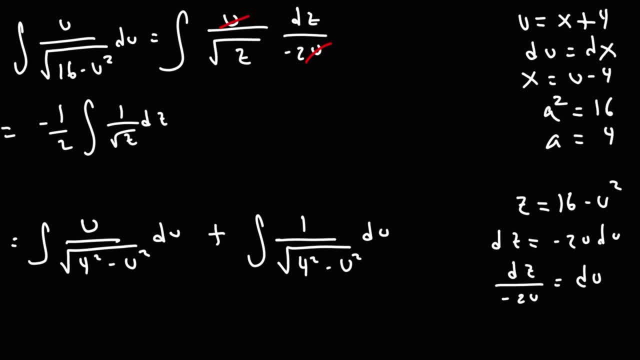 it will change from z to the positive half to z to the negative half. So we have this. So now we could use the power rule for integration. So add in 1 to negative 1 half. That's going to be positive 1 half. 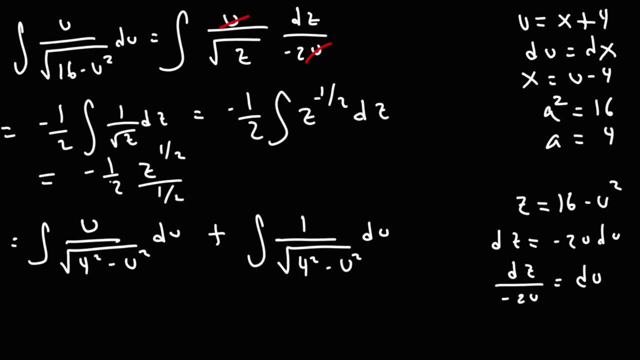 And then we're going to divide by that result. Now, 2 times 1 half is 1.. So these cancel. So we get negative z to the half, which is the same as negative square root of z, And we know z is equal to this. 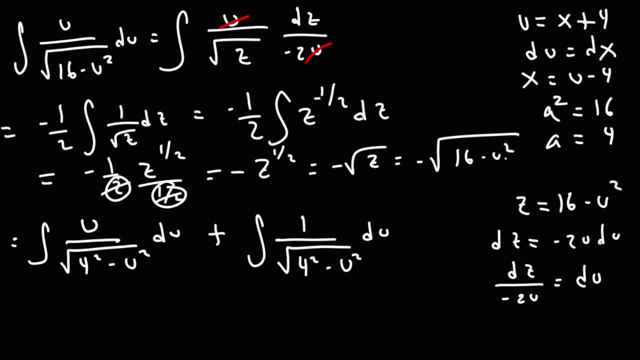 So this is negative square root: 16 minus u squared, And u is equal to x plus 4.. So that becomes negative square root 16 minus x plus 4 squared Now, because this is the result that we had after we completed the square. 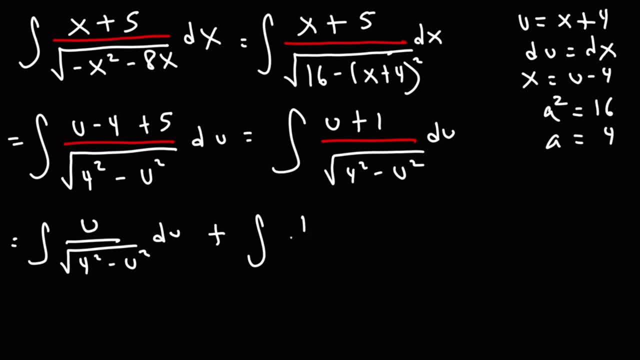 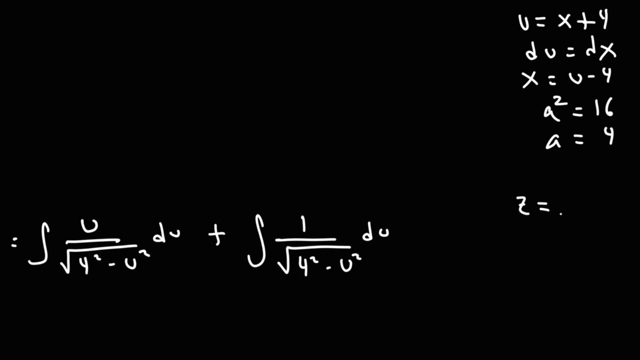 u substitution, integration technique, And for this one, this is going to be our arc sine formula. So let's go ahead and use u substitution on this. So let's introduce a new variable which we'll call z. So z is going to be 16 minus u squared, And dz the derivative of. 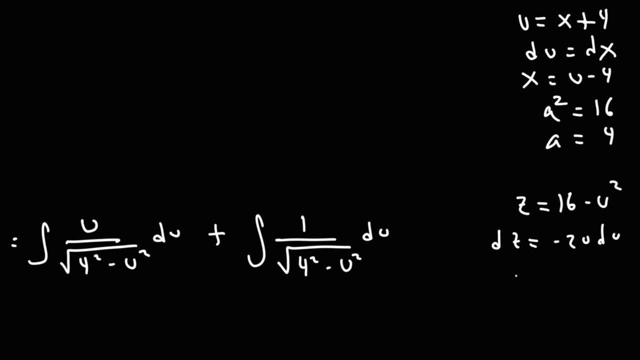 negative u squared, that's negative 2u du Solving for du. we get dz over negative 2u is du. So, focusing on this integral, we have this. So I'm going to keep the? u. I'm going to replace 16 minus u squared with z And du is going to be. 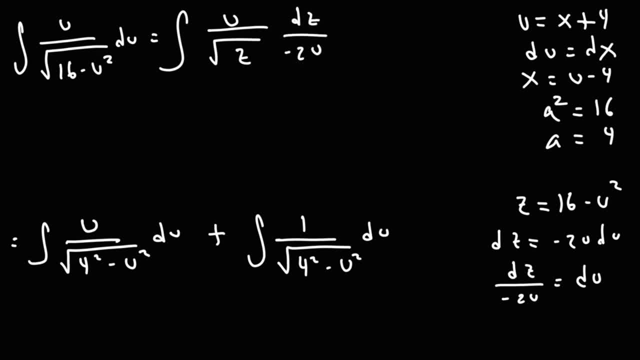 dz over negative 2u, So we could cancel out the? u and we could move the negative 1 half to the front. So we have this Now: z- the square root of z is z to the half, And if we were to move that z to the top of the? 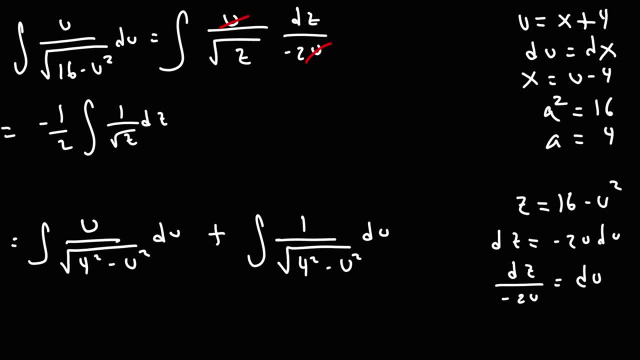 fraction. it will change from z to the positive half to z to the negative half. So we have this. So now we could use the power rule for integration. So add in 1 to negative 1 half. That's going to be positive 1 half, And then we're going to. 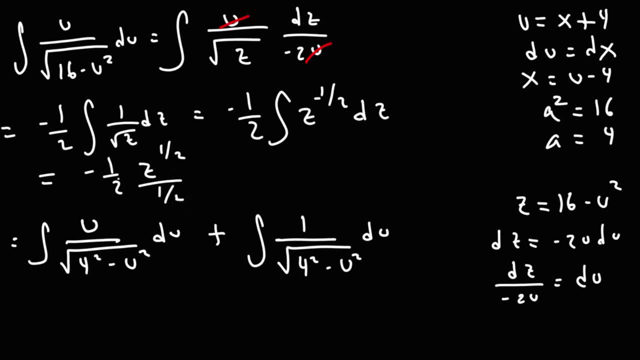 divide by that result. Now, 2 times 1 half is 1.. So these cancel. So we get negative z to the half, which is the same as negative square root of z, And we know z is equal to this. So this is negative square root 16 minus. 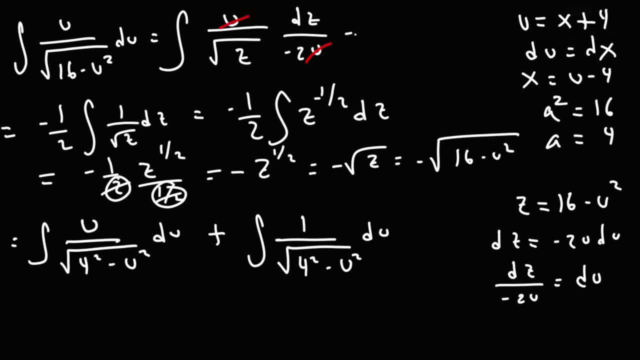 u squared And u is equal to x plus 4.. So that becomes negative square root: 16 minus x plus 4 squared. Now, because this is the result that we had after we completed the square, this expression is equal to the expression that we had in the beginning inside the radical, which was- I'm going to write it: